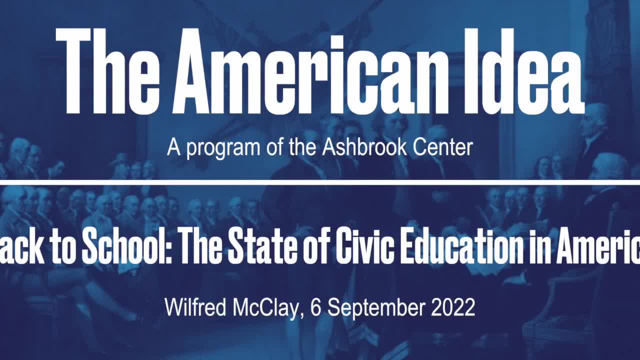 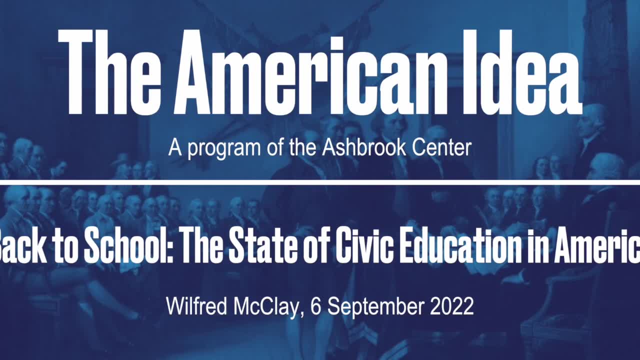 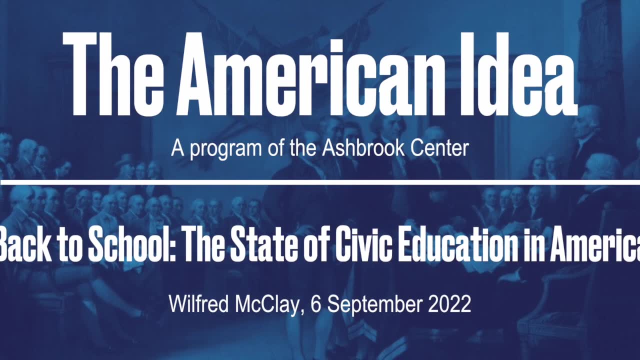 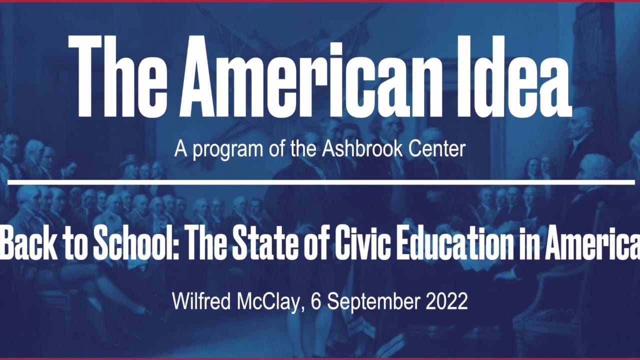 Hi, I'm Jeff Sikinga, Executive Director of the Ashbrook Center, and this is The American Idea coming to you from Peter Schramm's library in Ashland, Ohio. In this podcast, we explore America's crisis in civic education. Too many people today don't understand the history and 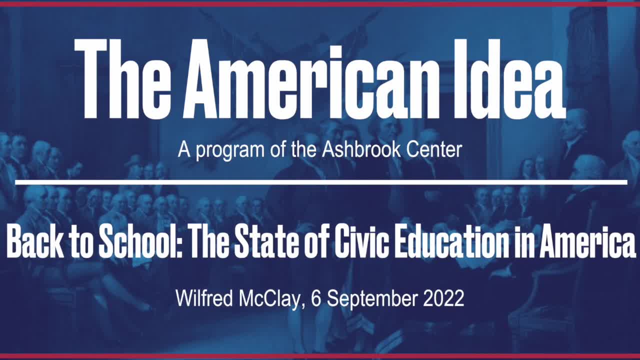 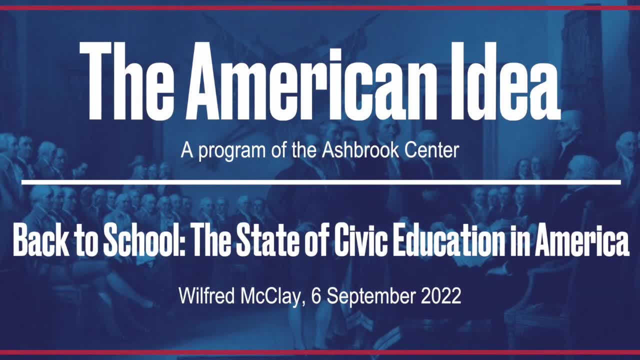 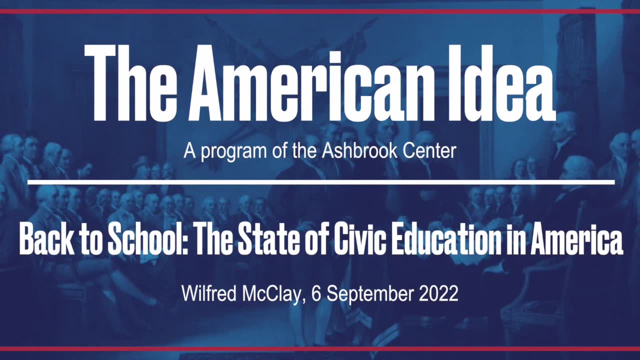 principles that make us Americans. So we're here to explore America's history and principles and what they mean for today, what we can learn from them and how we can restore them to their rightful place in our hearts and minds. We think it's the most important thing we can do as 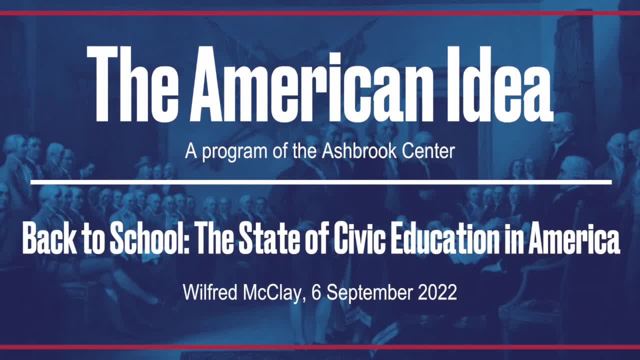 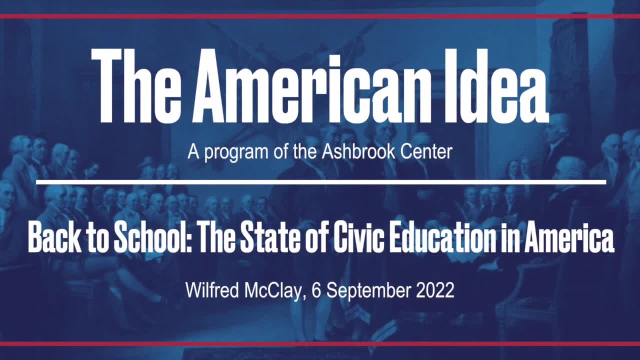 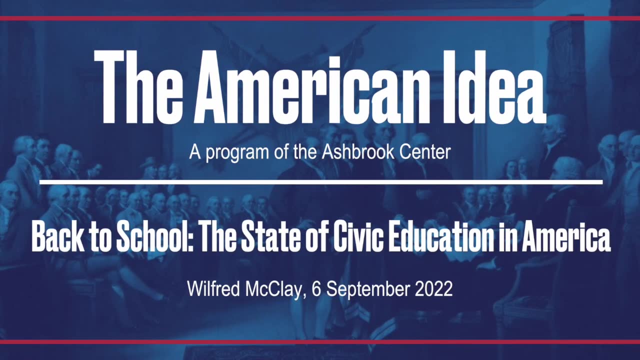 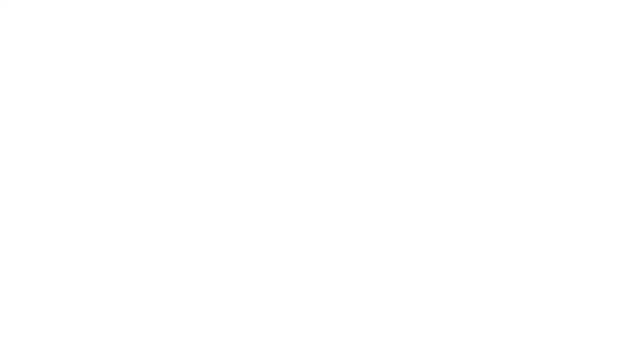 Americans to keep our experiment in self-government alive. So thank you for joining us in this important conversation. You can learn more about Ashbrook and the work we're doing with students, teachers and citizens at ashbrookorg. Well, I want to thank everybody for joining us this evening for a webinar. 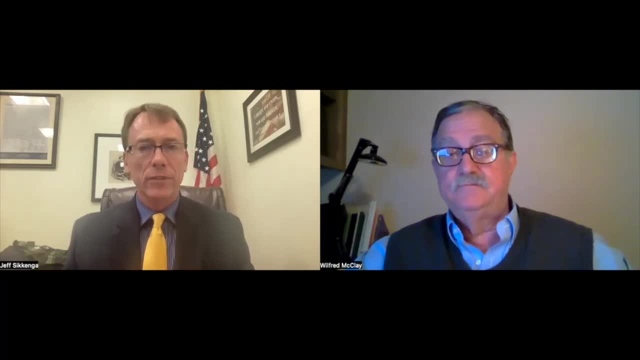 the Ashbrook Center's Citizen Webinar Series on Civic Education. For those of you who don't know, I'm Jeff Sikinga. I'm the Executive Director of the Ashbrook Center. and those of you who may not know the Ashbrook Center, we're an educational center located at 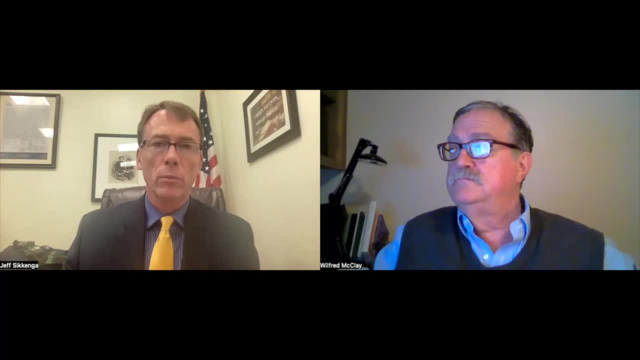 Ashland University in Ohio. We run programs for students, teachers and citizens both here at the university but also across the country, And our mission really is to educate our fellow Americans in the history and founding principles of our country And as an educational center. 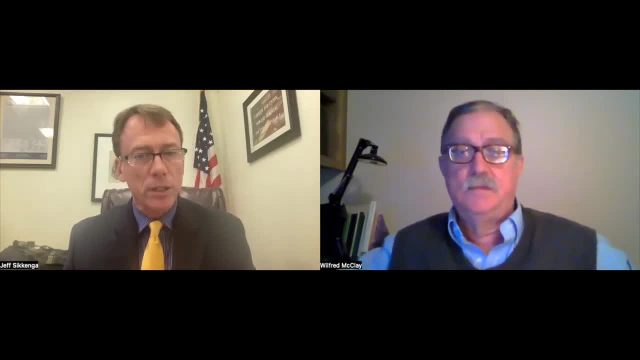 we really strongly believe that education is not about indoctrination, and not even really about information, but about discovery- discovering the truth for yourself. We try to root all our programs in Aristotle's old dictum that all human beings, by nature, desire to know. 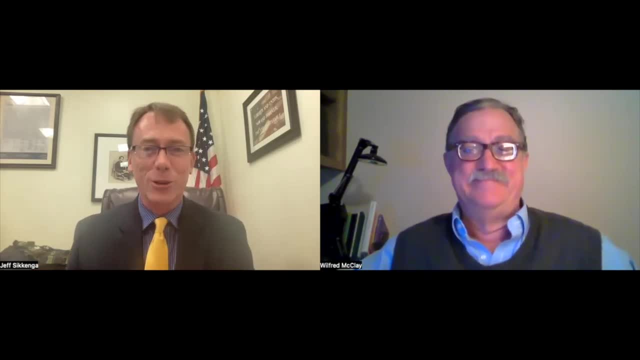 And then we add: but they don't want to be told, They want to discover it for themselves. So, and we found, the best way to discover for yourself is through conversation. So we want to have a conversation this evening about the state of civic education in America. 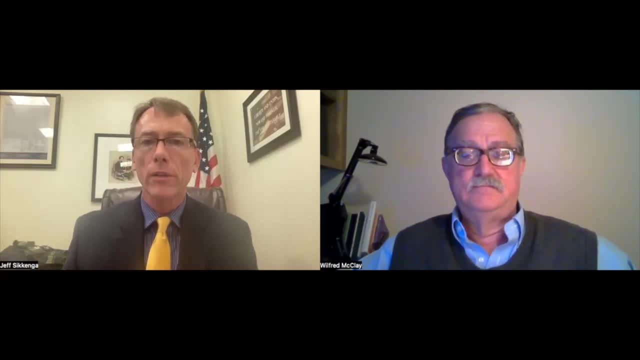 as students are going back to school. What are they learning about America? What should they be learning about our country? Join in that conversation this evening. Please feel free. join us through the Q and A function. You'll see it there on your screen. Delighted to have. 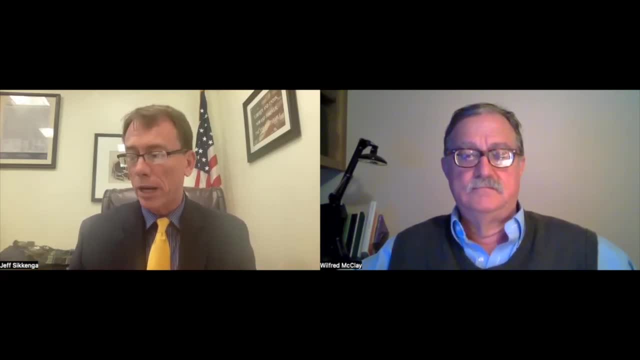 folks post questions. We'll try to get to as many of those as possible And for our conversation this evening I'm delighted and honored to be joined by Professor Wilford McClay. Bill is the Victor Davis Hanson Chair in Classical History and Western Civilization at Hillsdale College. 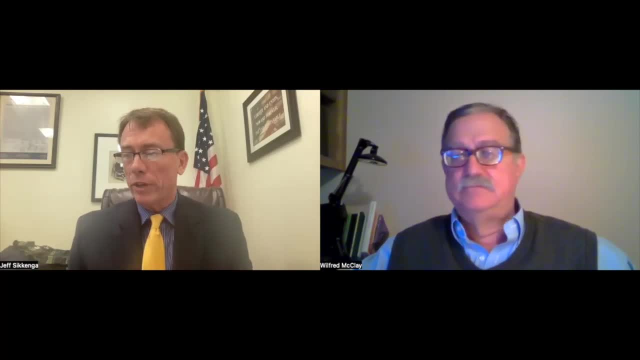 Before his current appointment, he was Professor of History at the University of Tennessee at Chattanooga and the University of Oklahoma And also has been the Ronald Reagan Professor of Public Policy at Pepperdine University in Malibu, California. He received his bachelor's from 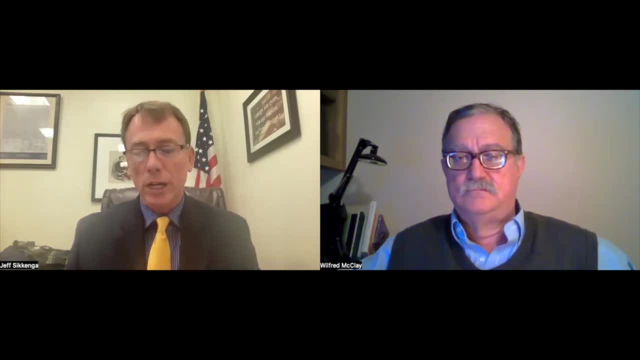 St John's College and his PhD from Johns Hopkins University. Bill is a terrific teacher, a terrific scholar, also a widely published author. Many of you may know his books. There are a lot of them, but just a few that stand out to me in looking at his long list of impressive works: The Masterless Self and Society in Modern. 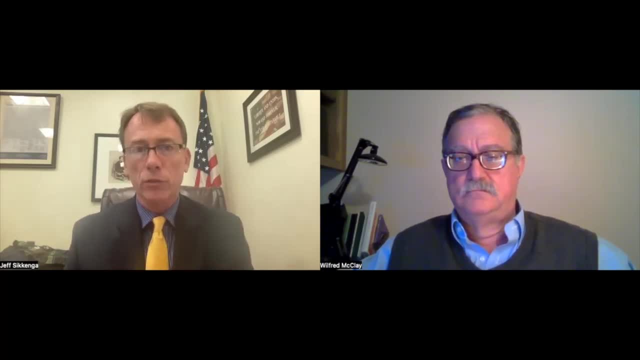 America, which won prizes in American history and intellectual history, A Student's Guide to US History published by the Intercollegiate Studies Institute, And also, most recently and perhaps most famously, of his recent works, Land of Hope, an invitation to the great American. 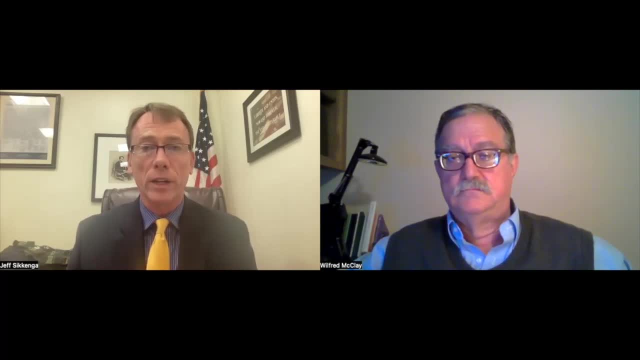 story which I just have to recommend to all of our listeners out there. It is a terrific, terrific work and a great service to the country and to the American tradition. Besides being a scholar and a teacher and a professor, Bill is also a member of many boards. 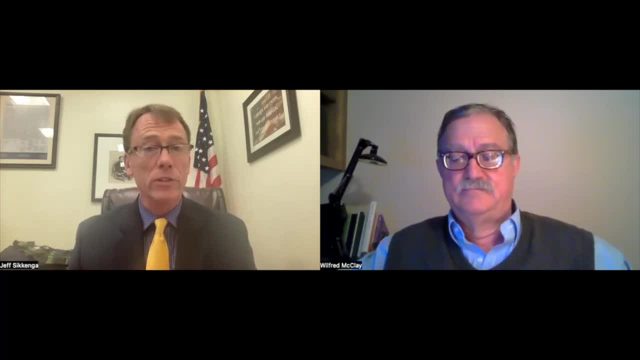 both civically and publicly. He has been past president recently of the Philadelphia Society terrific organization and also on the board of directors of the Ethics and Public Policy Center in Washington DC, And we at Ashbrook are really honored to have Professor McClay serve on Ashbrook's. 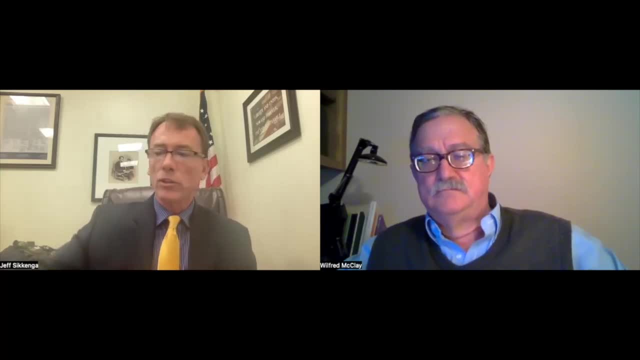 National Advisory Board on Civic Education, And it was actually in that capacity that he very graciously allowed us to republish an essay by him entitled Civic Education, Rightly Understood. So it's a real honor to have an expert in civic education and 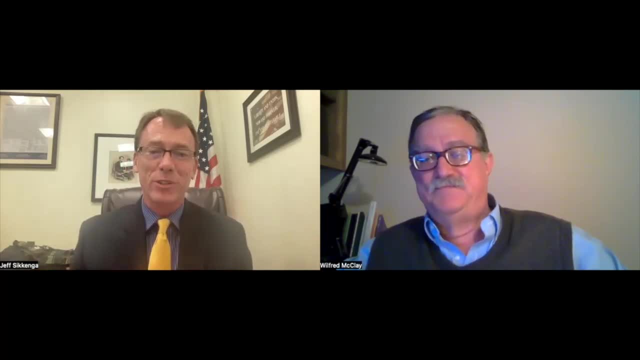 in this education in the meaning of America. Professor McClay, thanks for joining us. It's my pleasure, And I hope you don't hear dogs barking in the background. I'm babysitting three dogs at the moment. So well, thank you. We may have to get up and admonish them, but a lot. 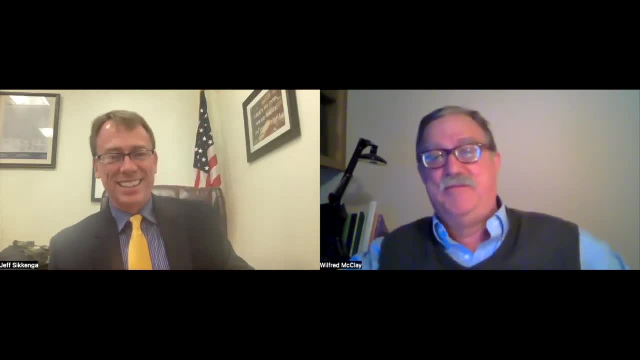 of good, that will do. Yeah, they need some civic education, That's right. You know, I was struck by your essay that you, that Ashbrook- republished on Civic Education. Rightly Understood, because you actually call civic education there. You. 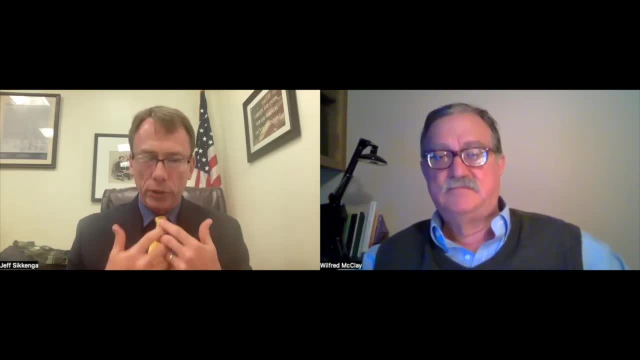 emphasize the importance of citizenship, of educating citizens, young people, to be citizens, not just the nuts and bolts of knowing how a bill becomes a law, as you put it. But you know a line that struck me and I just like your take on this. help our listeners understand. 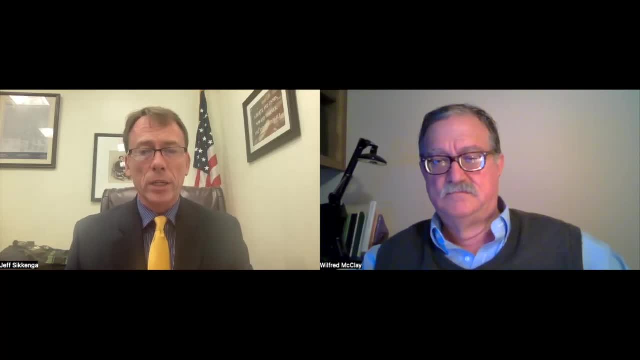 this a little bit more, especially those who may have read the essay already. You actually argue that civic education- and I'll quote you here- is as much a task of the heart as it is of the head. In fact, you even call it an education in love. Now, that's not how most people think of their. 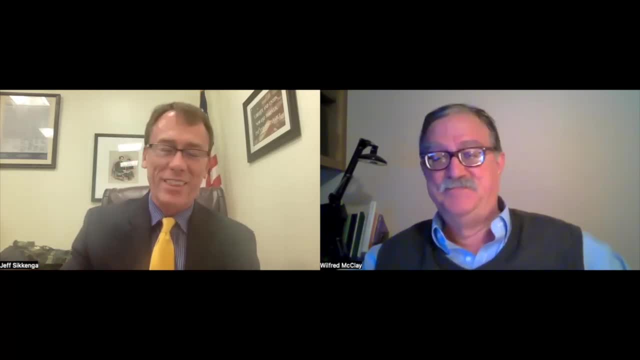 high school civics classes. What do you mean by that? Yeah, Well, an important part of educating young people about what it means to be an American, or really the citizens of any political entity, but particularly we're talking about American. we're concerned with America And with this quality of American citizenship. that 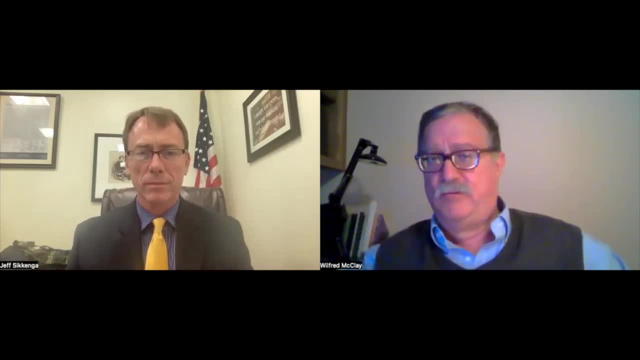 is open to dissent and to making up our own minds about things. Yeah, Okay, as you were so nicely putting it in the introduction. So we have to form young people in a way that they understand that dissent or disagreement or criticism- maybe let's use that word- 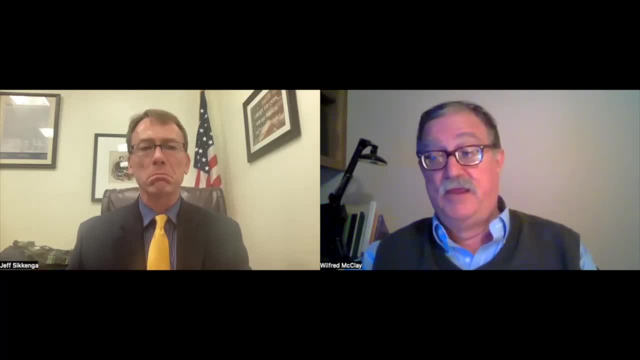 and love go together. That to love your country is not to be uncritical of your country. To be critical of your country is not to fail to love it. That those two things go together. And then it's the fact that a proper critical view 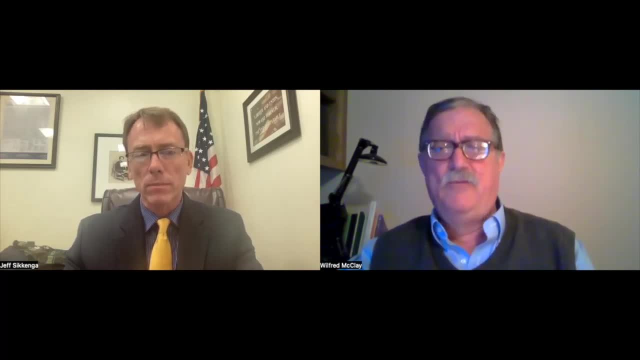 of your country goes hand in hand with the love of it, And it's really likely that when it's detached from love, when there's simply a kind of icy detached attitude, that you're going to make wrong judgments about the country to which you are connected. 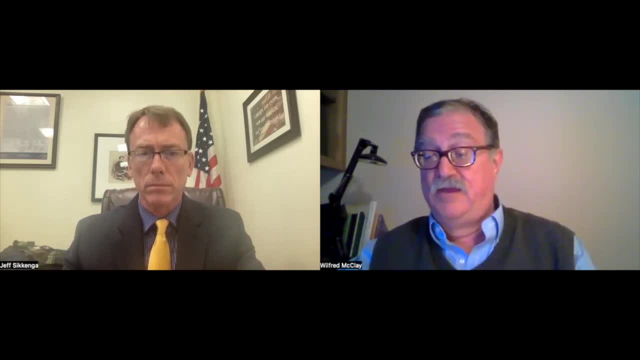 whether by birth or by naturalization, it is a part of us, particularly those of us who are born in the United States. It's something that comes to us, so to speak, with our mother's milk, But that to be worthy of that citizenship. 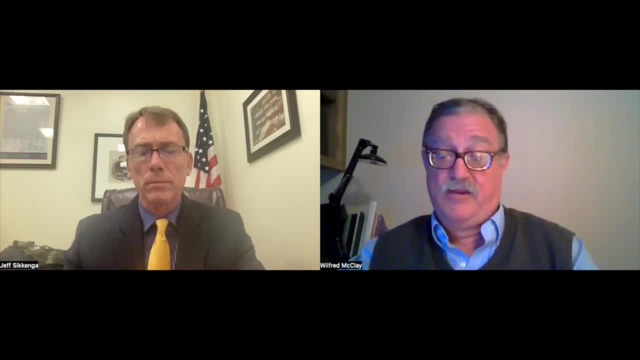 to have the right understanding of patriotism, of patriotic sentiment, is not an instinctive thing, It's something that has to be. It has to be educated, You know. it has to be refined. It can't just be a sort of gut level, visceral. 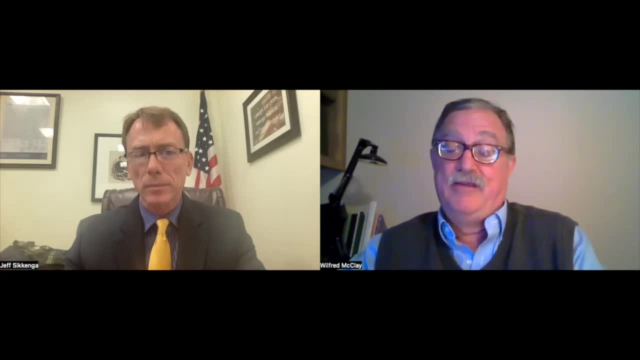 you know Yahoo kind of response. That's not enough to be a good citizen of the United States of America And I have to say, one of the things that goes with this is thinking again. this is just as unpopular as saying it's an education in love. 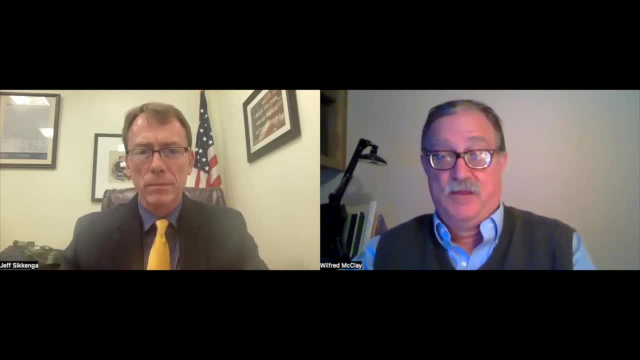 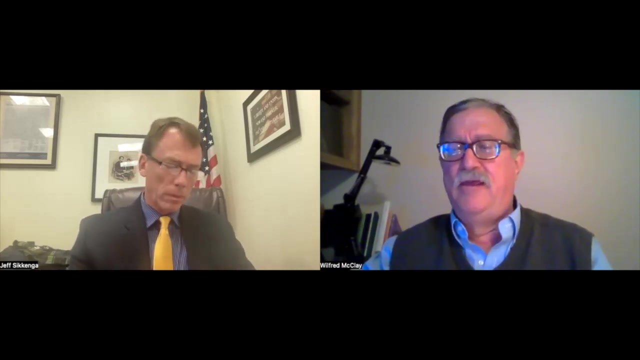 is that civic education is a kind of moral formation. I think we have shrunk from that idea that there's a formative dimension in civic education. It's not enough to instruct young people in how the system works, how a bill becomes a law. 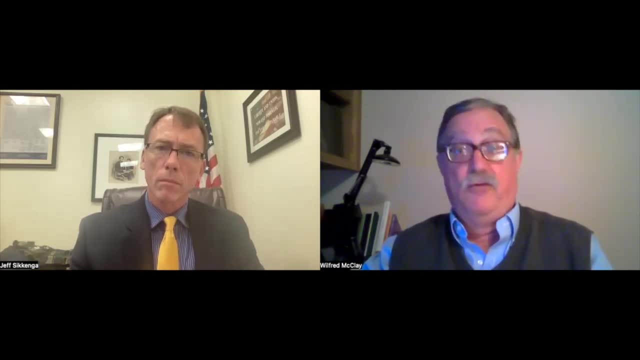 you know what our rights are, blah, blah, blah. I mean all those things are important, But one of the things we see today is that even in very well-educated young people, the graduates of Ivy League colleges- there's an absence of a certain kind of formation of the soul. 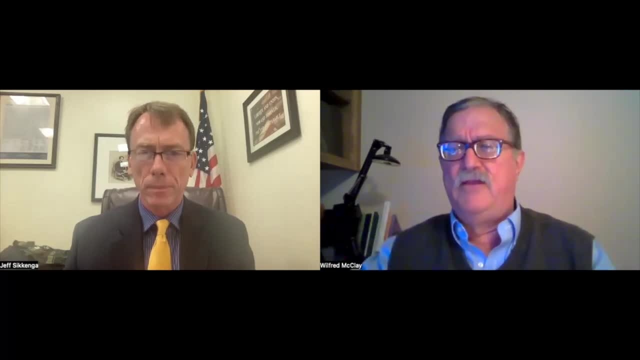 that accepts and understands and revels in the fact that we are a country, we are a culture that engages in dialogue, in polemic, in dissent, in argument, in deliberation, that we're deliberative. We're deliberative In our best. we should be a deliberative democracy. 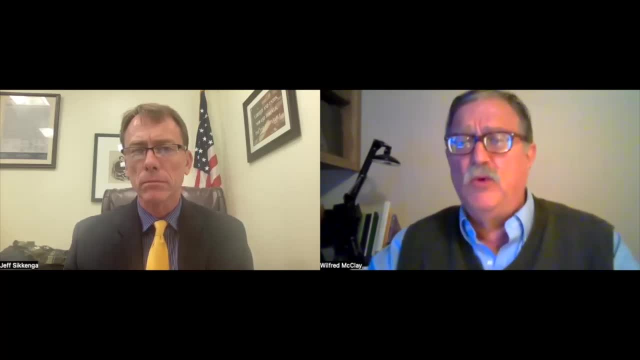 But to be a deliberative democracy, to have citizens who can talk to one another and listen to one another and understand the role of ideas, the right of ideas to exist that are very different from the ideas that one may hold oneself. This is a kind of discipline of the soul, isn't it? 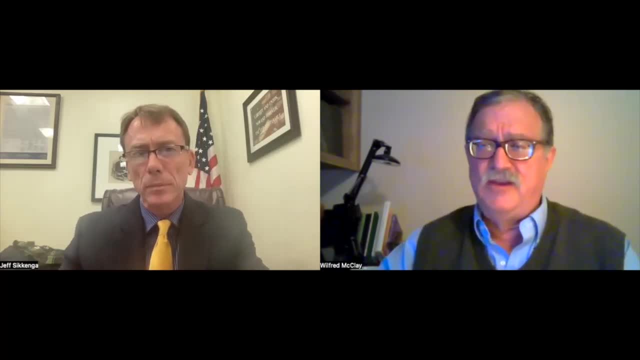 I mean, if you think about it, it's an education in a certain kind of deep regard for the opinions of others and a reluctance, really a forbearing from feeling that the only way to have things right is if everybody agrees, or anybody who disagrees just shuts up. 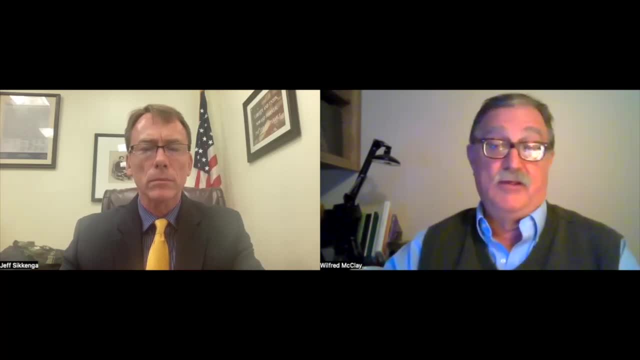 We've had experiences in our history of the right doing that to the rest of the country. Now we're having the left do it. I think for the most part Same problem. It's a very difficult thing to educate people to a society in which there's a give and take. 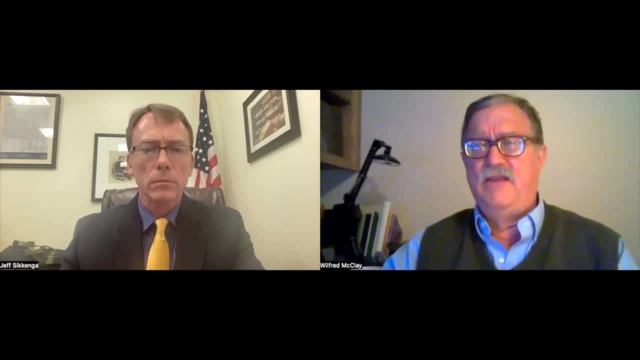 in dialogue and discussion and a recognition that in the end, once the matter is settled, we go on, and peacefully. We don't endlessly litigate issues. We find a stop, a stopping point, and then we go on and maybe we litigate them again in other ways. 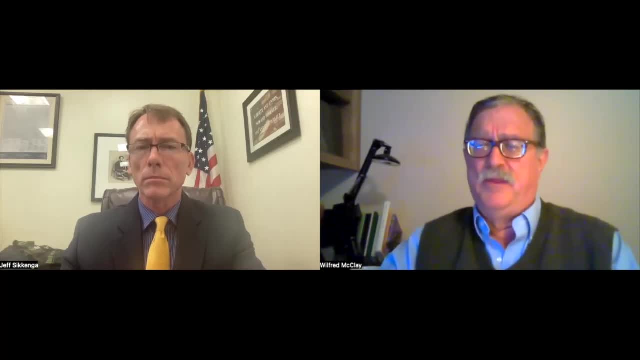 but we don't just kind of keep chewing on the same boat. That is something that I think we're losing. I think we're losing the idea that those who don't agree with us have a point of view that deserves our respect and it deserves our listening. 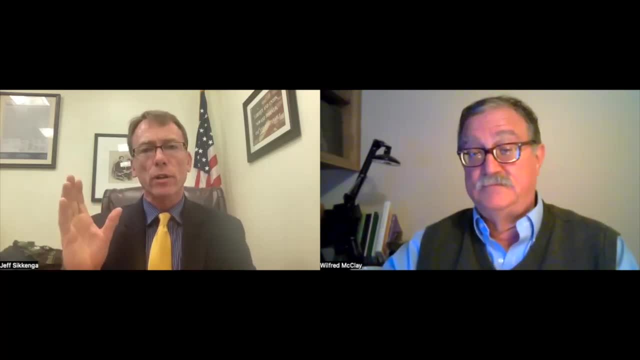 Fascinating. I mean really that's interesting what you say. Civic education sometimes is thought of as just boosterism, Just the love part, just blind love, uncritical love, Seeing everything is perfect in that you know sort of romantic way. 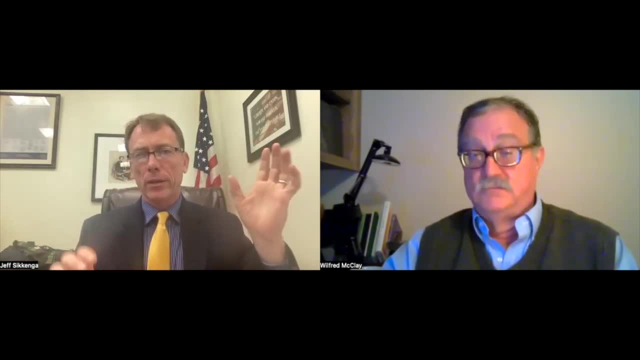 But then the other part is criticism. right That sometimes we civic education is in many ways nothing but criticism. And the way that you actually put it in your essay- I think you call it: students are being taught the inglorious story. 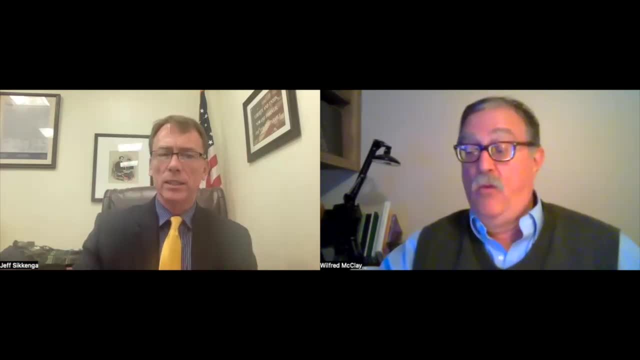 Yes, right, What do you mean by that? Well, yeah, simply that it's. you know, I just finished doing an online course with a colleague here in Hillsdale And it was very interesting. We did a sort of spontaneous summing up. 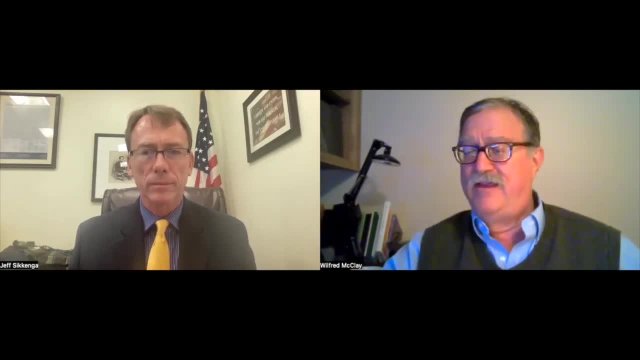 discussion And my colleague felt it really necessary, in a way that I found kind of jarring, to say at the end: well, of course we've committed horrible crimes and sins and this and that, but we're in the end we're really not so bad. And not that I actually disagree with the 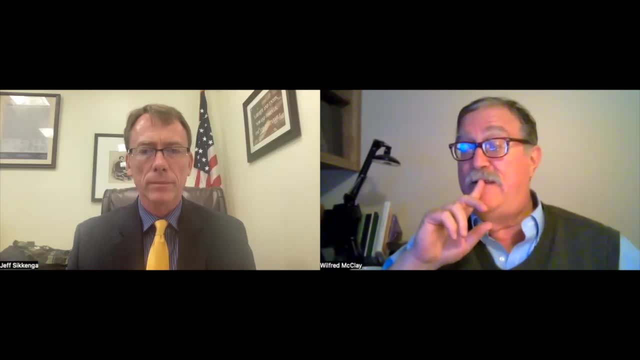 content of that, But it was done in a way that struck me as- and I guess I'm criticizing my colleague here and I don't really want to do that- But that it was done in a way that was sort of a reflex. we're developing a reflex that to apologize for our failings, which are many, and 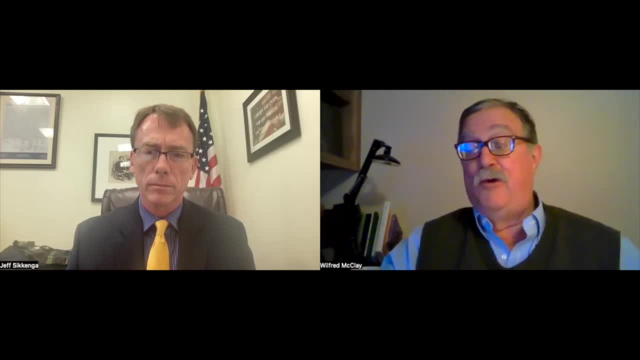 genuine. You know, it's the only way to to avoid, for a nation state to avoid, those kinds of failures is to attempt nothing or to attempt very little. And we've attempted much, we've been audacious as a country And we've had many, many more successes than failures. Failures are. 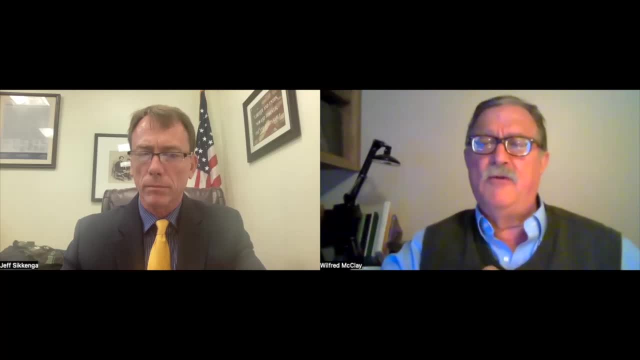 particularly heinous because they go against our creedal assertions about what kind of people we are, And I think it's painful. I think we need to confront that. that should needs to be part of civic education. But to to ignore or give short shrift to the magnificence of our history, to the, to the many astonishing, 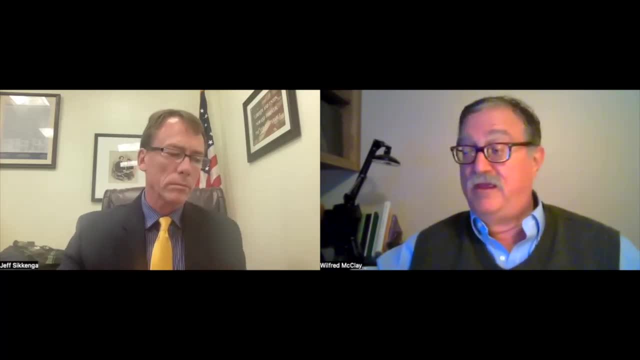 things that we have done in, in particularly in the 20th century, I think in the latter half of the 20th century, the Second World War being prime among them- And to fail to give credit to those things, to give emphasis to those things, is, I think, an even 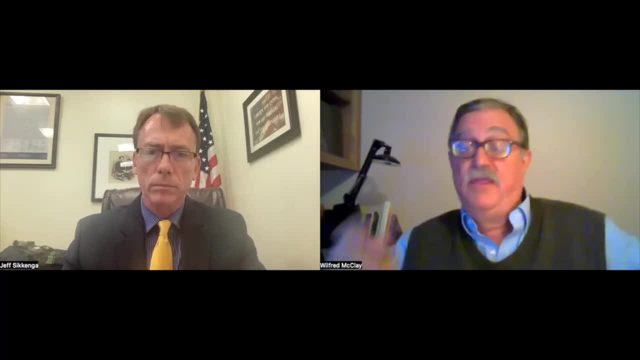 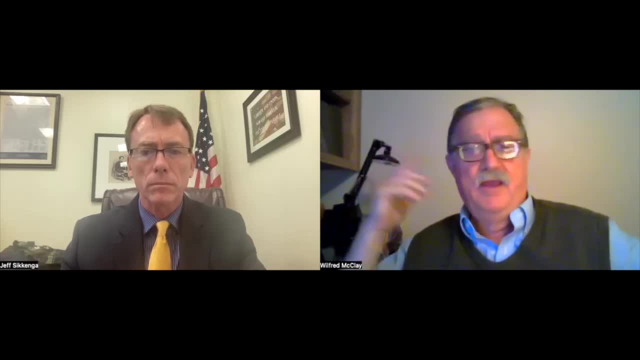 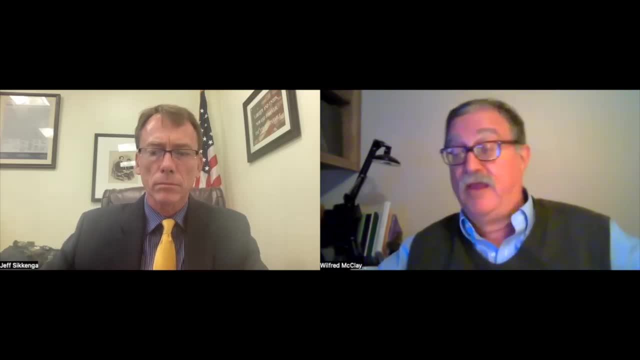 see, and which, by the way, is part of the reason I wrote Land of Hope, is that I wanted to provide an alternative. But if I were a young person seeing my, the country presented in such a negative light by, you know, historians and others who have a bit, or they're very conscientious people, I know. 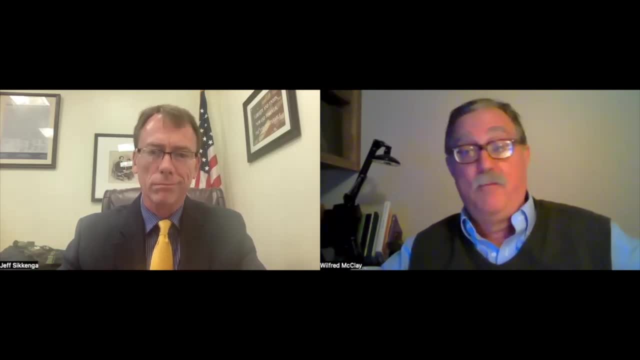 these Because they're very conscientious people. I know these people. i've lived all my work, lived and worked all my life and they're not bad people. they're not really. they're not interested in destroying america for the most part. but i'll ask them. 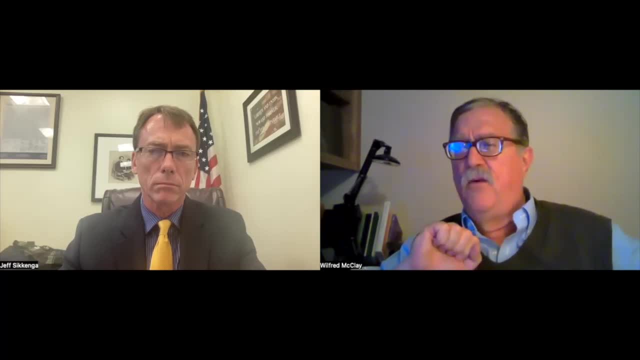 i'll ask my colleagues and friends: um, what do you think the cumulative effect of a of a whole career and a whole department of history at your institution? not true, at hillsdale, by the way, but, but, uh, other places i have taught it is true. what's the cumulative effect of all of that? 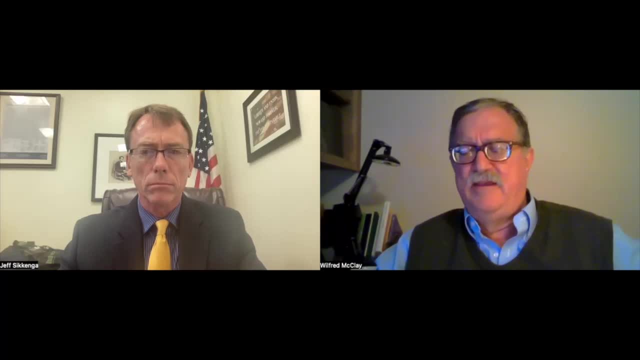 being presenting a, a fundamentally negative and apologizing view for our national history. and you know what they all say: it's the same thing. they say: not my problem, not my department, not my job. my job is to is to follow the evidence, is to be critical. uh to uh. use the best practices of the, of the, the professional training that i received. 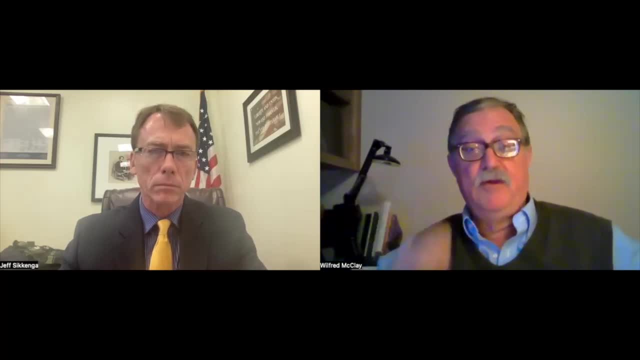 and that is what is the mark of superior historiography. um, it's, it's, uh, not a wrong answer, but i think it's very myopic. it's, it's, there's no. um, there needs to be a kind of hippocratic oath or something to the effect that. 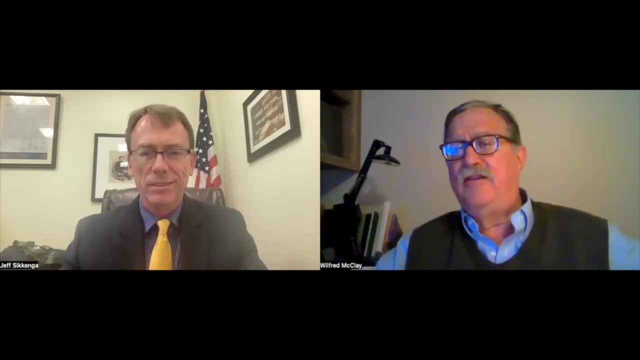 of taking into account what the effect is going to be of all the debunking and and and. think about what kind of general and overall image of the country it is coming to the minds and hearts of young people i i think of. i have a friend named harry ballen who i always 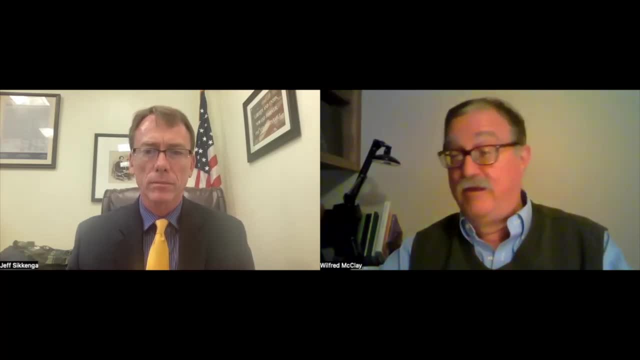 feel i should credit him on this- that he's a lawyer in new york, but he has many, many interests. and harry said to me once over breakfast. he said: you know what i'm going to do, i'm going to do what i'm going to do. i'm going to do, you know, i think- and actually this was while i was writing- 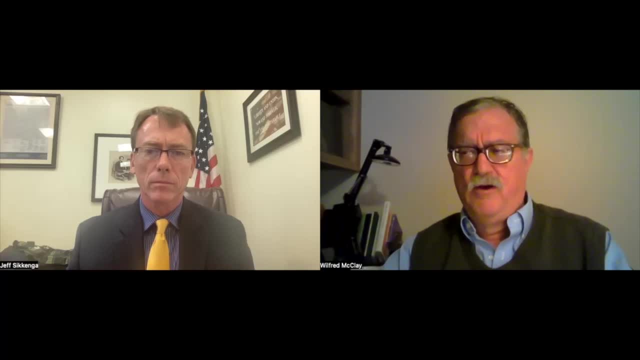 he said i think for young people to grow up in a country where they're taught uh, where they come to believe that they live under a bad regime, it's damaging to their souls. and at first i thought he was being kind of grandiose. whenever people start talking about the soul, you know you, you do kind of 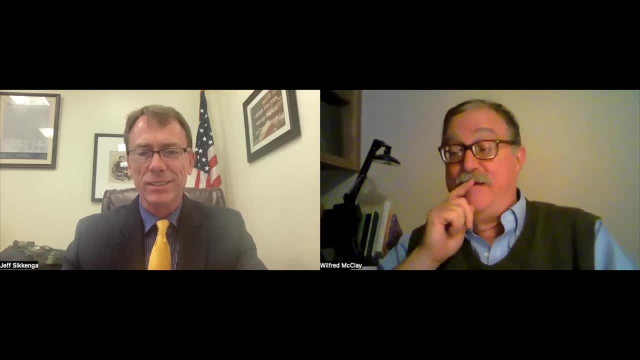 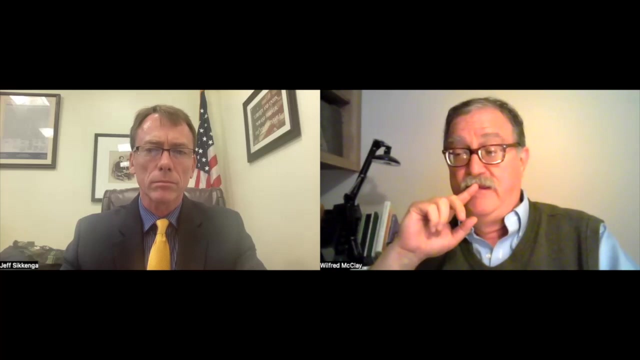 what, what is there to wait a minute? but um, the more i thought about i thought he he was putting into very simple language something very profound that i think we've lost. it's a sense that what, um, what? what we teach is about the nature of the regime that they live under, the society they live in. 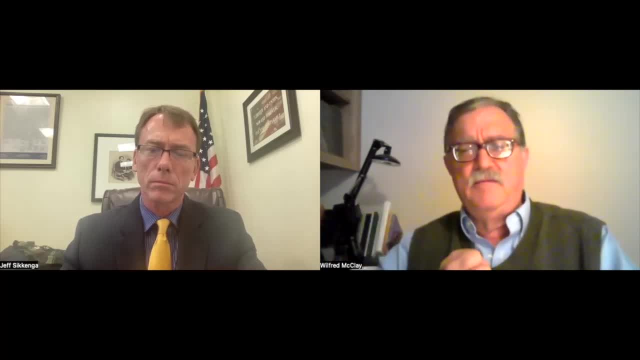 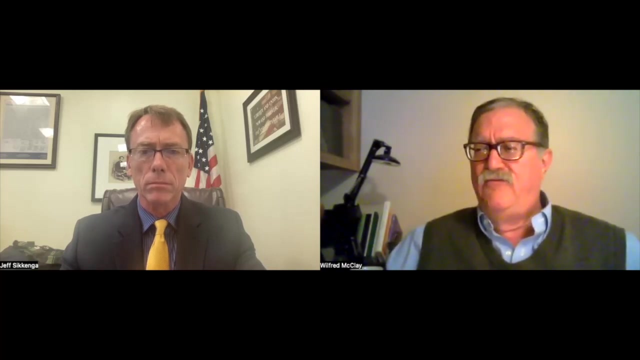 um, is it fundamentally bad? is it fundamentally bad or is it fundamentally good with bad aspects? and you know, that's the kind of judgment that actually a young person does make. um, is this fundamentally, uh, something that i cannot trust? i cannot pledge my allegiance to that. i'd want as much as possible to see myself as being apart from detached from, alienated from. 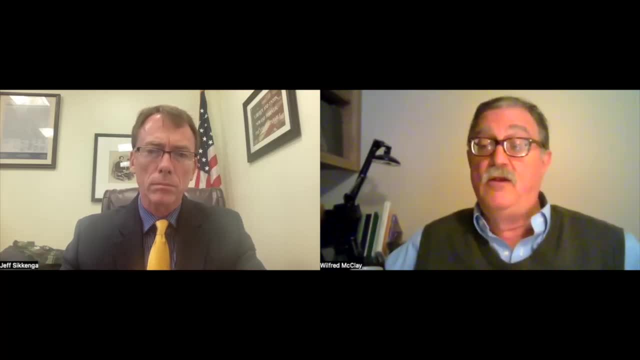 even, and uh, or do i want to take up the challenge of membership in this society? uh, of a full membership in it, and uh of um, doing all that i can, both by way of assimilating what, what is known about the past, and taking that heritage as my task for my own life. 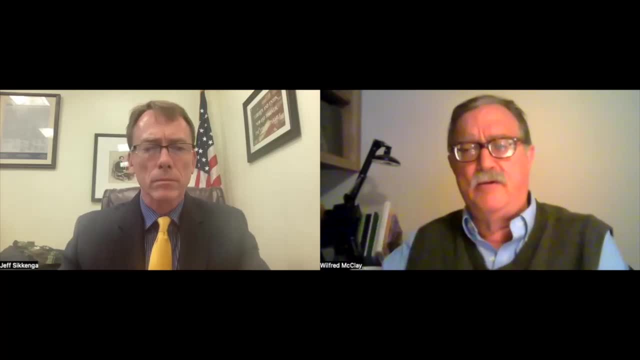 to take what i've inherited and make it better. that's, that's the way to go, uh, that's and that's. i think a part of that's a part of civic education, as much as teaching people about um, the, the uh electoral process, the difference between 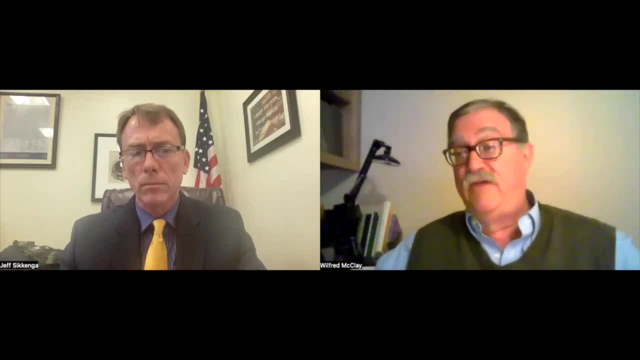 the three branches of government, etc. all the things you think of when you think of civics. i think those have to be done. i think a modicum of american history has to be taught. it's very important. i think you can teach the principles and i'm going to sound like a historian. 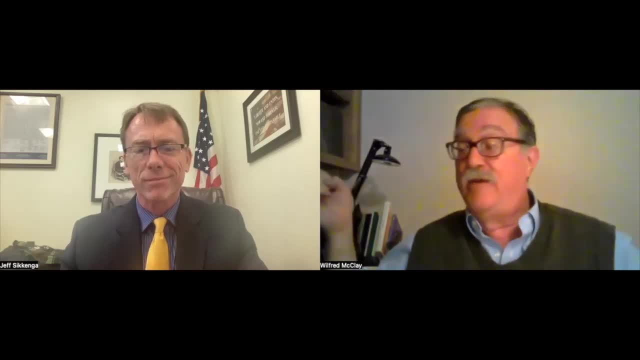 here. but i think you can teach the principles of separation of powers and checks and balances and all that. but if you look at the historical evolution through, let's say, the 17th century and uh and uh, english slash british political evolution, you begin to see why, um, those kind of safeguards are important. we're. 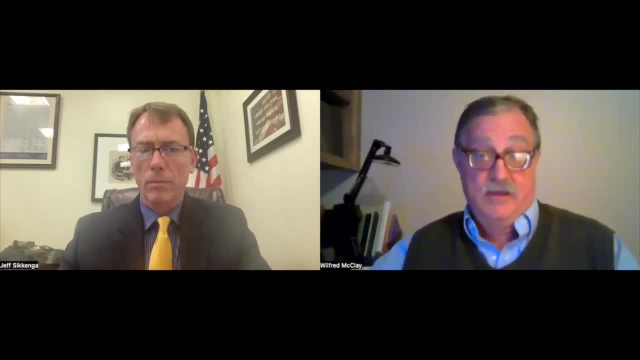 living through a time now which leading scholars- two guys from yale and harvard law school- published an article in the new york times saying we ought to junk the constitution. i think this is a very short-sighted view and ill-informed view. it's very presentist, to use a term that people like to use this very. 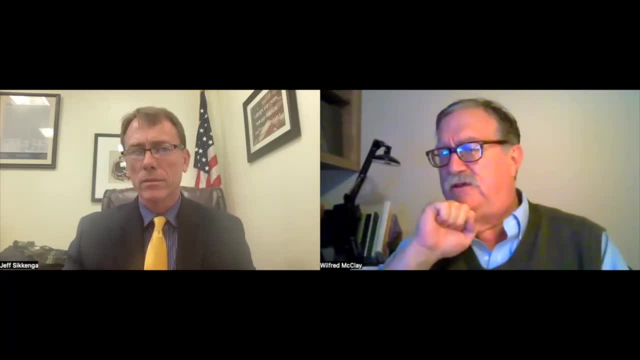 present. mind you know, we don't like the supreme court decision, we don't like, uh, the electoral college, because it keeps electing the wrong people. um, therefore, uh, we're going to, you know, simply eviscerate the constitution. um, you know, there's all sorts of examples of constitutional amendments that the people, uh, you. 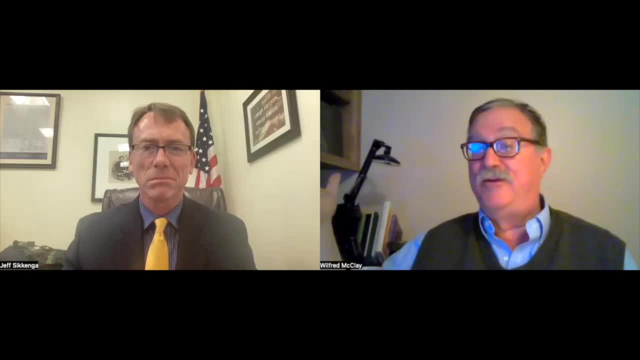 know who press those. you know the limitation of the president to two terms. uh, the republicans might have liked to have had that one back in the reagan administration, but you know, uh, that's, one of the reasons you don't tinker lightly with the constitution is that you think through what. 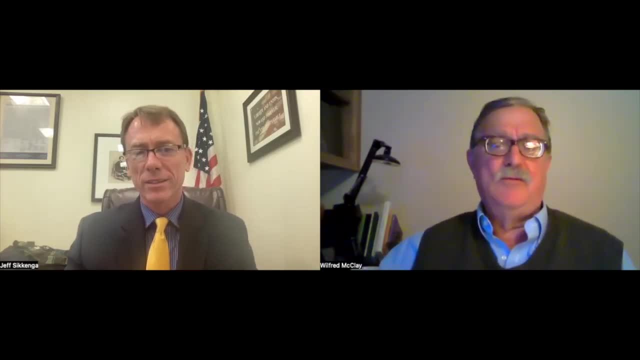 what are the general effects, not just what you can get in the short run. so so, anyway, i think that they. i would just say, finally, that i think actually a certain reverence for the constitution- getting back to the issue of love, um, is requisite. madison thought this, and you and jefferson, of course. thought, yeah, you should change everything. i have a revolution every 15 minutes and change the government every 20 years. yeah, all kinds of things he would say, uh in his letters. um, even washington did not expect george washington did not expect reagan uh nevada to be reelected. she became the. memos in that independent member. yea, he's being reelected again, true, now, um, that was, that's a little later. the canadian겠어요 has been a battle with the international opposition, as i, as would say sometimes that's um, but that's when it was in fact that that was the only time canuff turned out is away from. expect the constitution to last. it should have it be around 230 plus years, and counting would have astonished him. i think this is a great achievement and i'm not not, uh, something to be taken lightly, because the principles animated constitution are sound as ever, particularly about the dangers of the concentration of power. um, but we see this all the time. so you well, you. 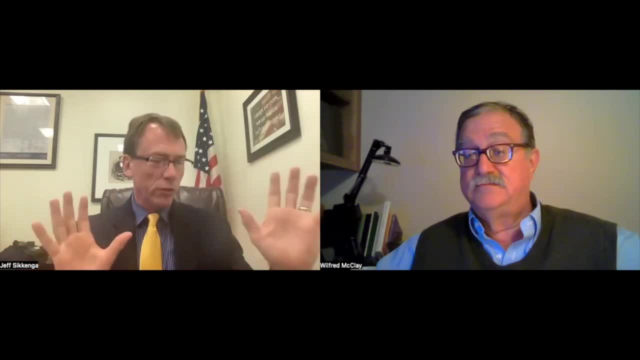 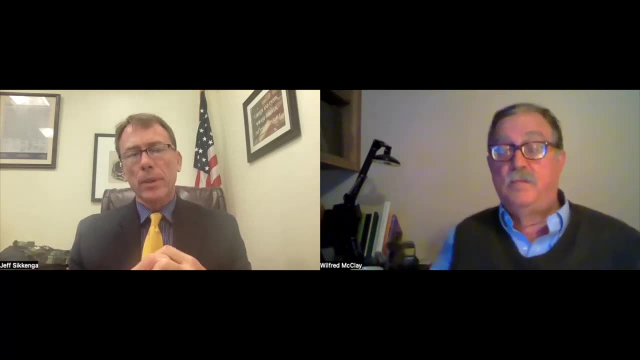 mentioned, though, thinking about again, love on one side, criticism on the other, and and putting them together in the right way, informing the hearts and minds of young people. um, honest historians, your friends and colleagues in the history profession who, as you say, might not be intending to destroy america, but they are- um, they're not thinking about the effects of their 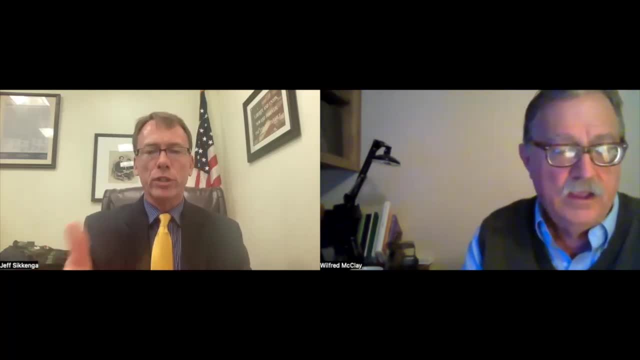 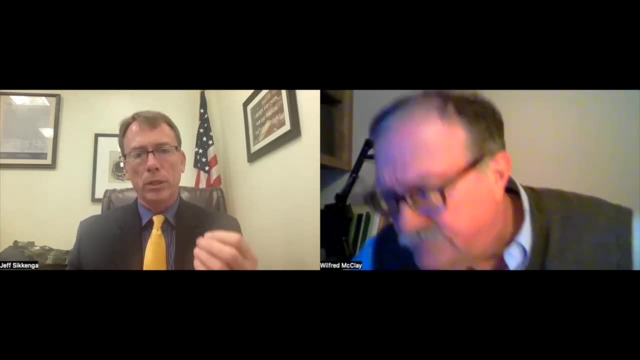 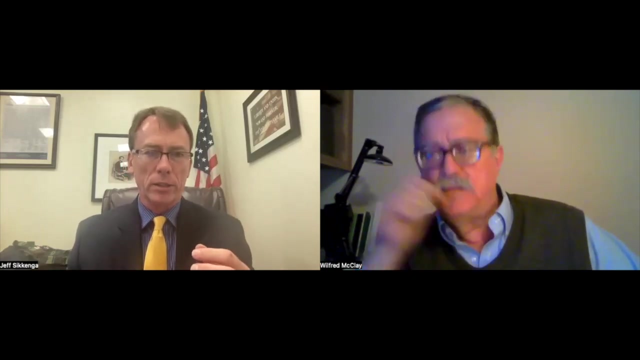 continual, uh, merely critical approach to teaching young people. but then it, what about others? take, for example, probably the most obvious public in immediately today. important example of that kind of critical approach to america, the 1619 project, um, is: would you consider that also honest history or is something? oh no, and look i, i don't know any. 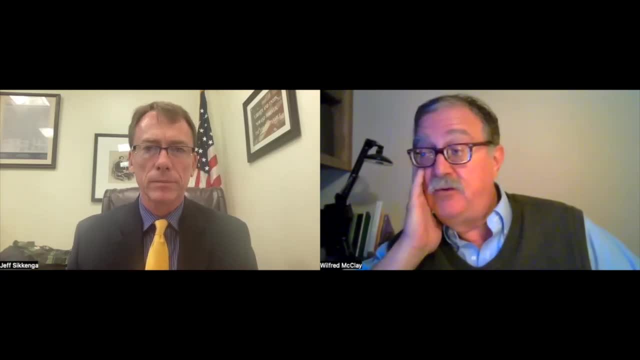 respectable historian who, um would defend the 1619 project as as good history? i maybe there is. maybe there is one, but certainly certainly uh. several of the people i most respect in the historical profession, uh, who are none of whom are conservatives, um, uh immediately came out said: this is outrageous, this is not um. uh and some of 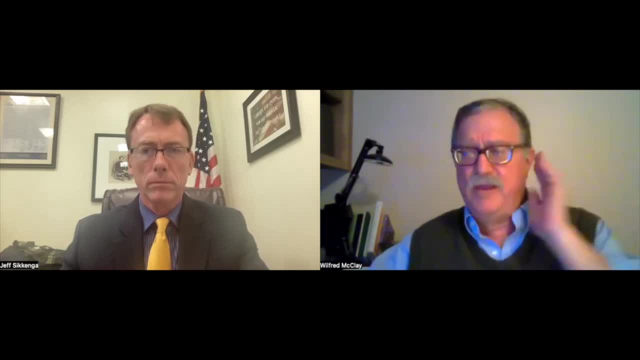 the. you know that i don't want to get into all the ways that this has been a kind of dishonest undertaking. they've even edited uh, surreptitiously edited uh copy on the website. as for the fact that this has been a kind of dishonest undertaking, they've even edited uh copy on the website. as for the fact that, 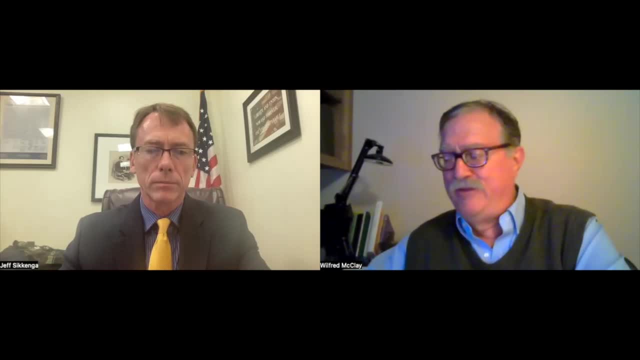 philip magnus has found out, uh, through some amazing detective work. um, it's a journalistic project, that's. that's the bottom line. nicole hannah jones, the the mastermind behind this, i think uh, either herger or jake silverstein of the new york times, but uh, 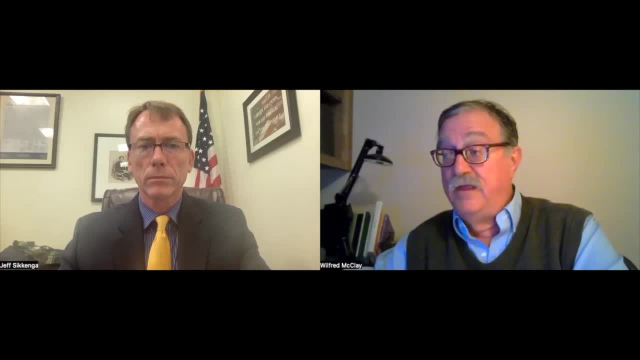 uh, the mastermind behind this, i think, uh, either herger or jake silverstein of the new york times. conscience ground the uh uh, but um uh uh. she said as much. she said we. we didn't really think of this as of like a revision of history. we thought of as a way of saying let's read the work. 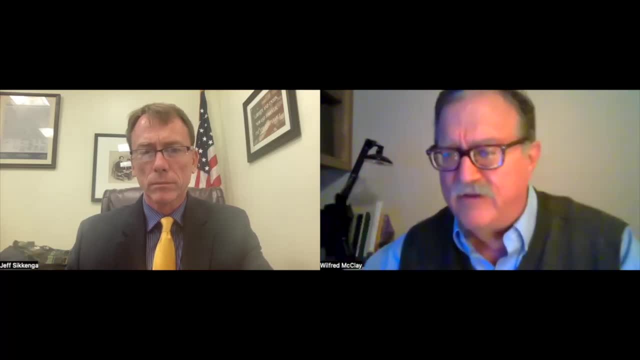 saying: let's reimagine the narrative of the historical narrative. uh and uh. what if we began with the idea that the introduction of slaves into what would then later become the united states um in 1619 at jamestown, that that that's the real beginning of american history, not just the 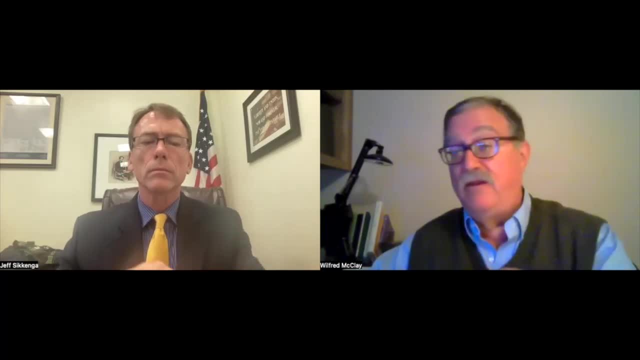 beginning. it's the founding, it's the true founding: um it's, uh. and that the foundation of american history is the oppression of slavery, of uh, of bondage, of chattel slavery, uh, um it, it's, um it's. it's an audacious thing, and then not in a good way. i think it's been: uh it's. 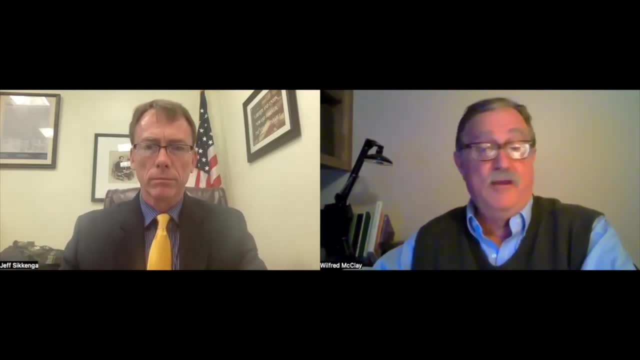 it's going to be leave its mark for a long time. there's a lot of free materials that the pulitzer center people are putting out that you know, reflect this perspective and, um, and really they have not been answerable for it. i mean one of the 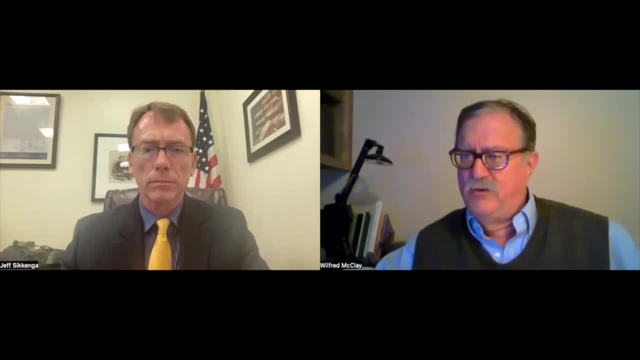 things we historians do. we don't do it as well as we used to, but we do. at our conventions and other venues we, uh we are forced to defend ourselves to, to answer our critics: uh, the times have never done, they've never condescended to do that, um, and i think it's pretty obvious. 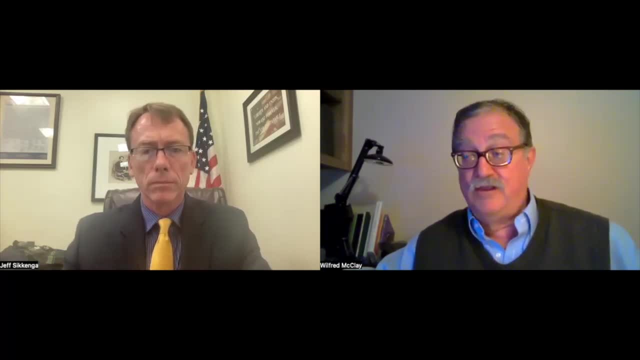 why that there's too much about the project that's indefensible. but let me defend one thing about it. okay, to surprise you. um, yes, that that well, i, i think, the idea of having a commemoration, a recognition of the 400th anniversary of the year 1619, which is what 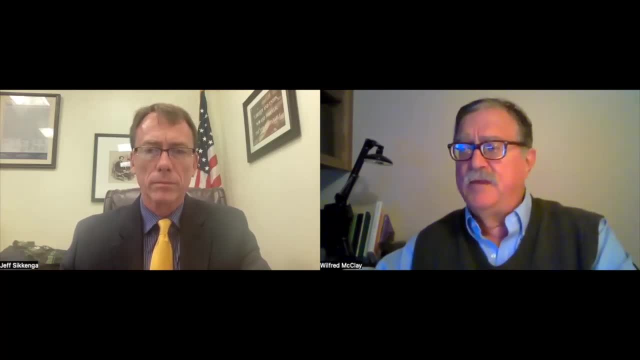 this all happened in 2019. um, i don't think that was a bad idea because, uh, i think, um, i'm thinking of one of the my favorite passages in in um wed du Bois's souls of blackfoot- wonderful book that everyone should read, and the chapter on the Sorrow songs, that is, the spirituals. uh, what we used to. 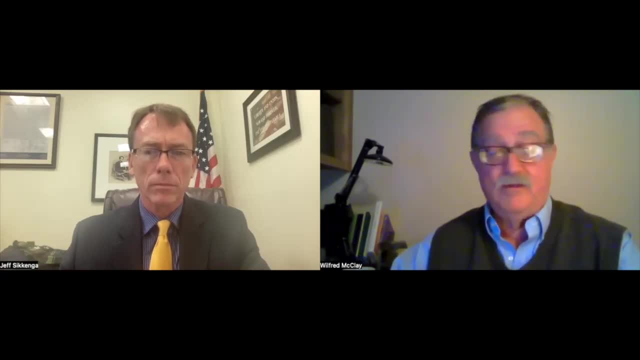 call the Negro spirituals, uh, in in a previous, you know era. um, uh, you know, nobody knows the trouble I've seen go down Moses, Etc. um, it's a wonderful treatment of them as an expression of the of the emotional and spiritual life of a captive people, um, and he sees it as a great 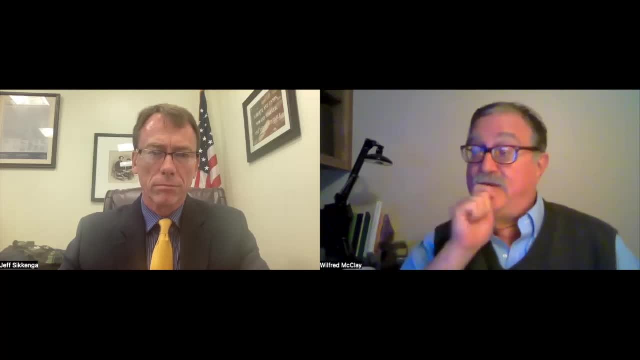 contribution to american culture. he says at one point the following: you know, um, what? you know? what would america be without its its black, without its african people? and he says: you know, before the mayflower arrived, we were here. and that's 1619, is one year before 1620. so, yes, uh, i. 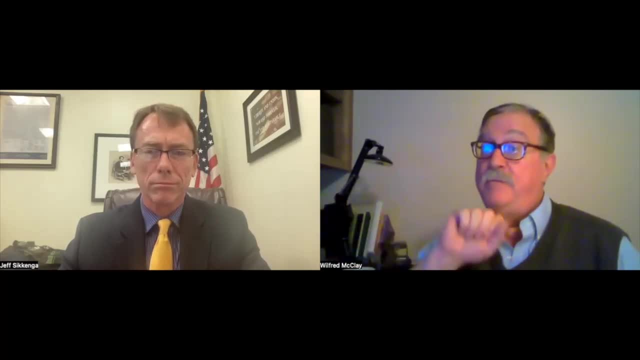 and i i think that's an important point. that could have been the point made by the 1619 project. it could have said: look, africans in america are not a sidebar, they're not just a kind of little fluky thing that happened on the side. um. 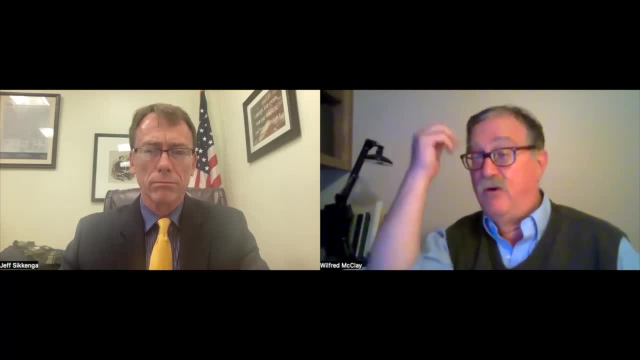 um, they are. they are part of american history and always have been, from the start. uh, david hackett fish has just published this amazing book, african founders, which i think makes something of the same point. it's going almost completely unnoticed. i'm going to do a review of it and 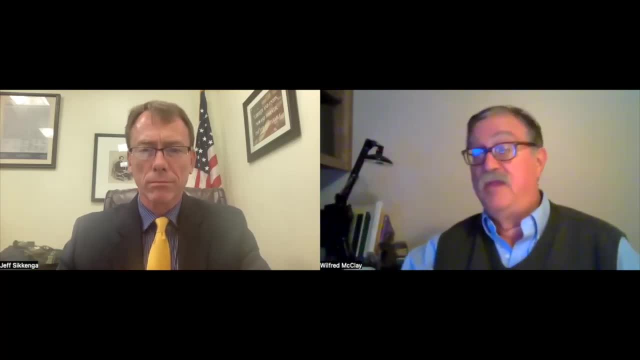 alan gelso has done a great review of it, and so, um, we'll get some word out about it, but it's because nobody wants to hear it. nobody wants to hear the atmosphere of 1619 is to accentuate the negative. to say: anti-black racism has been part of our national DNA from the beginning. um, well, you know. 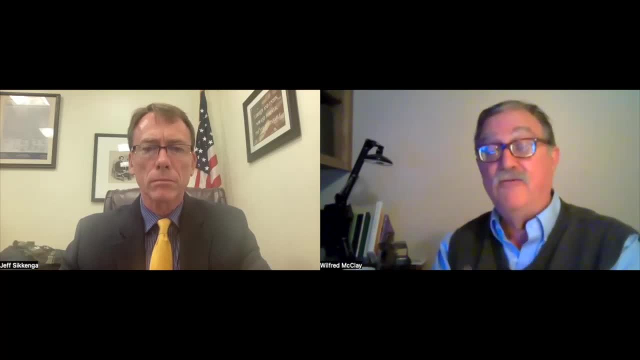 uh, uh. there's a- i think there's a lot of evidence for the contrary proposition, that africans in america have always been central to what america is and and, yes, we, we could write our histories better, um, if we did a better job of recognizing that and acknowledging it and and making that uh uh. that's the of the khoffman of africa. Praise theían. yes, we see this as a just a single matter of fact, um, from actually understanding the unknown and as of our assumption that was taken into consideration, that there's one thing that's not true- and i think it's true- confirmed that africans have been recognized for their tradition as national research. today we know that we got a great deal of artists and flourishes and or somewhat the kind of the opposite work, among them VIC. 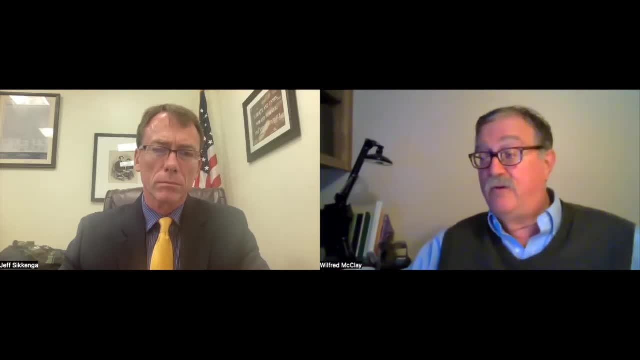 thematic aspect of what we do. I saw today that the college board is going to do an advanced placement test now in African-American history, And I have done nothing except read the New York Times' article about this, so I'm not particularly well informed. but I don't think this is a 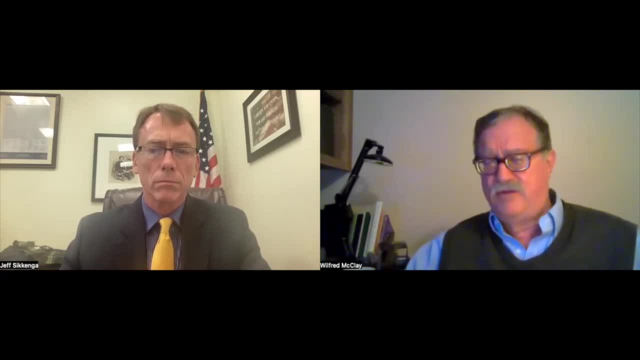 particularly good idea. I think it enforces, it reinforces the sidebar, the idea that African-American history is something apart from American history. And you know it's a close call. really I can see the merit of it, but I also then, can see the merit of any other large ethnic group. Let's say: 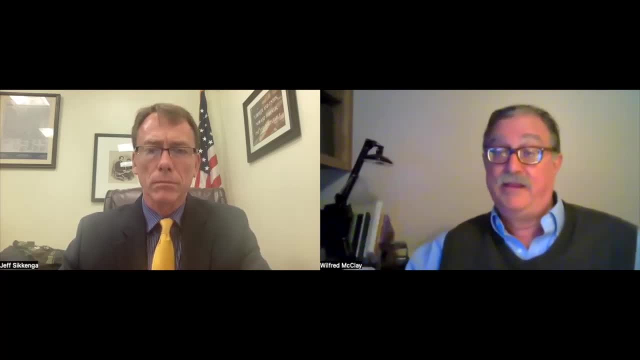 Catholic history Big. You could do a lot. You could do a lot with that. Have an AP course in American Catholic history- But that's not going to happen. The political stars are not in alignment to do that, But I think so. I think that getting 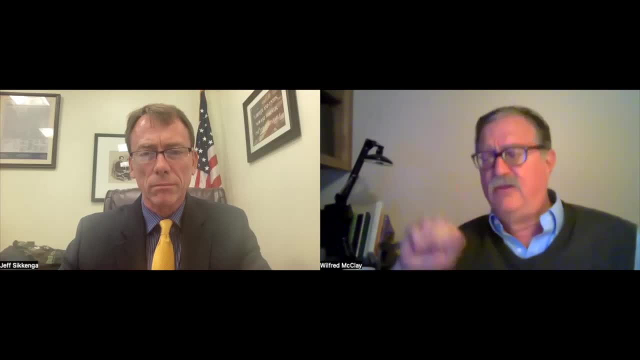 back to 1619,. I think we could have. there's another way that 1619 could have been emphasized, and that is that it was not only the year of the first enslaved individuals being deposited in what would be Catholic history, but it was also the year of the first enslaved individuals being become the United States in Jamestown. It's also the year that Virginia created the first representative legislative assembly, the House of Burgesses, a remarkable development in the history of American self-rule, of self-government, of self-governing institutions, of institutions. 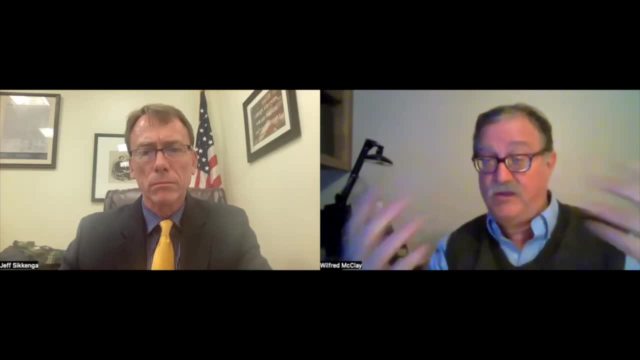 built on the notion of the consent of the governed, which would figure so prominently in the language of the Declaration of Independence. Both of these things happened: The introduction of enslaved people, who did not stay enslaved by the way. they became indentured servants because there was no provision under the 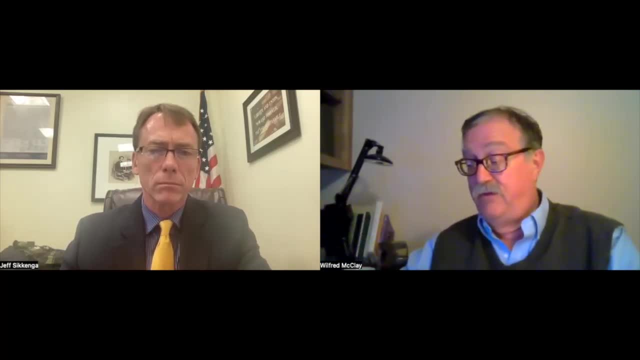 English common law for slavery. It was. it would be a number of decades late before slavery as a legal institution would come to Virginia, And it's a shameful part of our history. but it didn't happen immediately- 1619.. Anyway, you have these two different strands of the history of American. 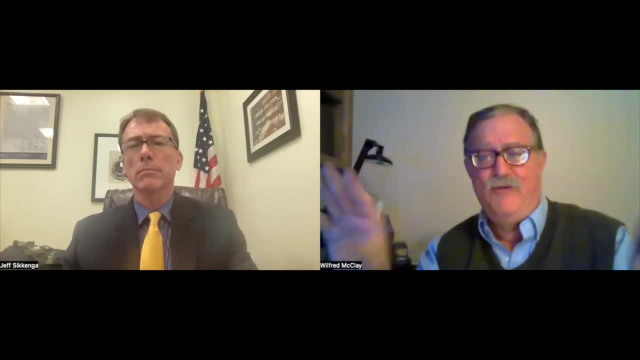 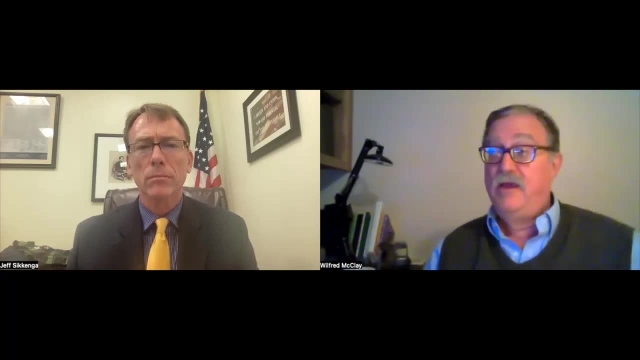 self-rule. two different strands, two different doorways into the future open, And one of the doorways, frankly, is a doorway to the past, to the long history of the domination of the strong over the weak, over the kind of lawlessness that had governed the institution of slavery and its 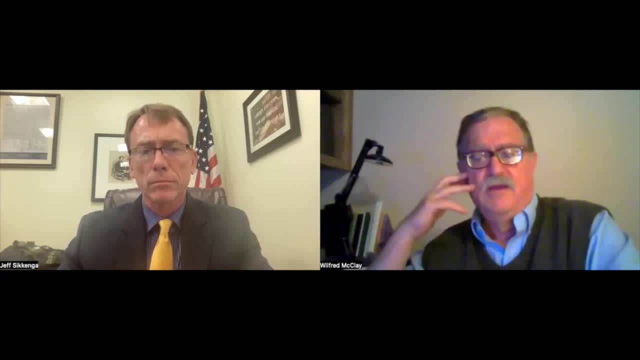 cognates for all of human history. You know the Caribbean was full of slavery when Columbus arrived. He didn't invent it, Americans didn't invent it. We invented anti-slavery. We have the first anti-slavery organization in the world, So it's a complicated story. 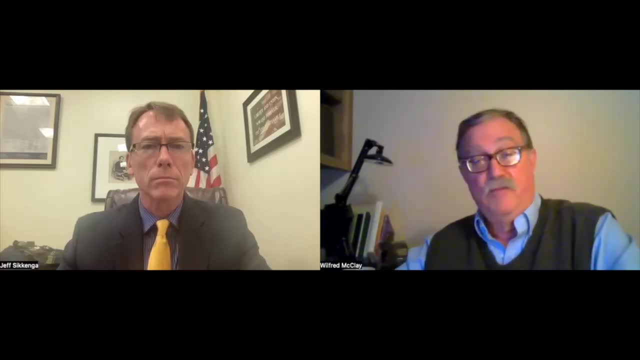 and it's not without many blemishes, And those blemishes should be acknowledged. But I think in the end I don't even say that teachers should all celebrate, end up celebrating American history. That's what I did. I don't think Other people may come to other conclusions, but you've got to be fair. 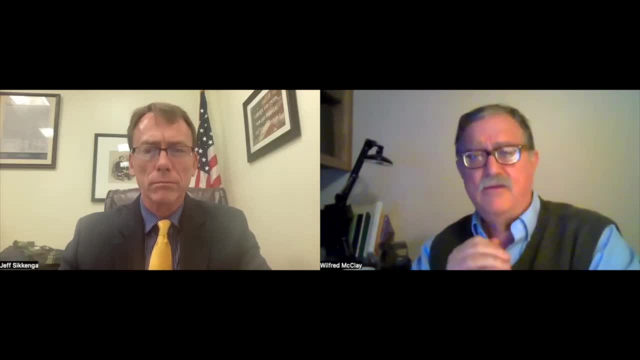 You've got to be fair and acknowledge the greatness, the great achievements, And you may think that they came at too great a human cost. Fine, Make that case. But make the case, Don't simply assert it, as I think is so often the case. Don't present it as an assumption. 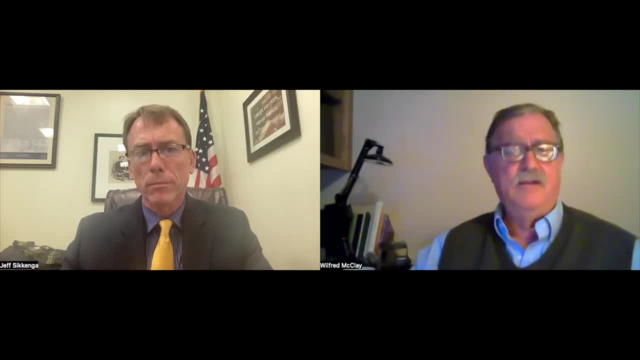 And don't do young people the service of telling them none of the things that are admirable about their nation and its history and the structure of its institutions. So in thinking about this combination of criticism and love- critical love, as you said- I was struck by one of the things in your essay where you 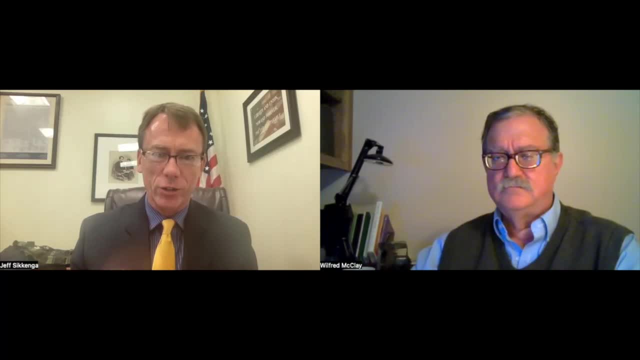 talked about Abraham Lincoln's civic education, which is pretty interesting given the fact that Lincoln really had almost no formal schooling. certainly never went to college, He read himself, but he really had no benefit of a teacher or any kind of organized educational system. 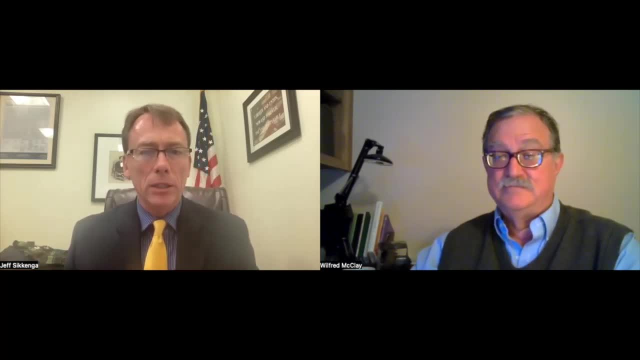 almost whatsoever. But you talked about Lincoln's reading of stories, in particular Parson Weems' stories of George Washington. Tell us about the kind of education that Abraham Lincoln got and how it shaped his American heart and mind. Well, that's a great question, And it does. There's all sorts of things that 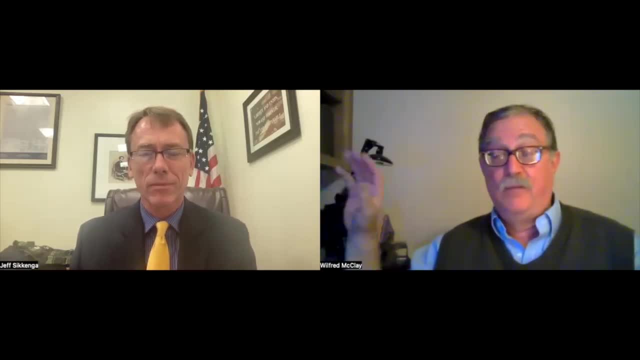 come out from it, including the fact that maybe our schools are really- I won't say unnecessary, but they're definitely falling down on the job In comparison to a man like Abraham Lincoln, who admittedly, was a little engine of ambition as his law partner. 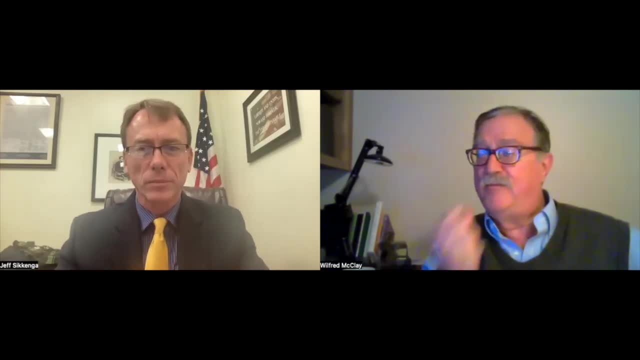 he was, as you said. he was a extraordinarily driven man, but he had virtually no formal education, And he was. He educated himself through his reading. He read everything he could get his hands on. Of course, it's well-known that he read all of Shakespeare's plays and had certain 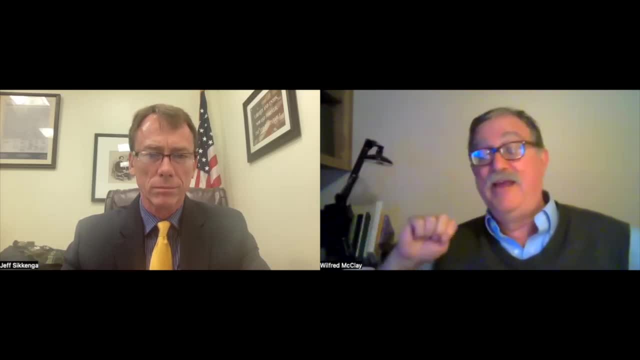 favorites like Macbeth- a good play for a political leader- And And the King James Bible, the effects of which you can see in some of his truly magnificent speeches toward the end of his life, end of his career. The cadences, the sense of the syntax, the word choice, the weighting of words. 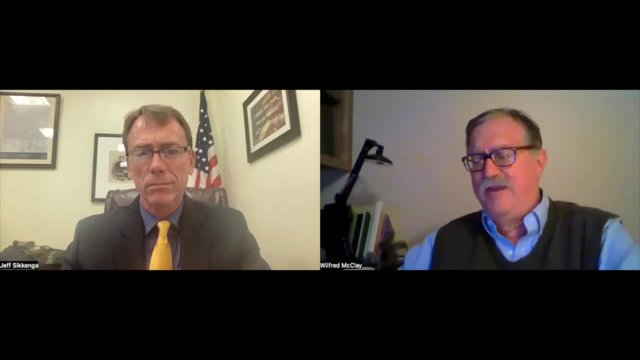 It all is so redolent of the King James Bible and of Shakespearean English. So Lincoln had, he had a, in a way, a superior education because he didn't go to school, Although school boys- and they were mainly boys at that time- did study those texts. 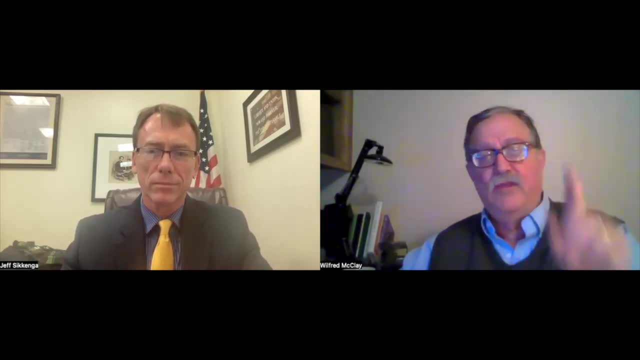 Anyway, the thing that I point out in this article that I think you're thinking of, Jeff, is that Lincoln didn't read much history. He read a lot of literature. He read, you know, all sorts of things Having to do with the law and political issues, but he didn't read a lot of history, as a young man anyway. 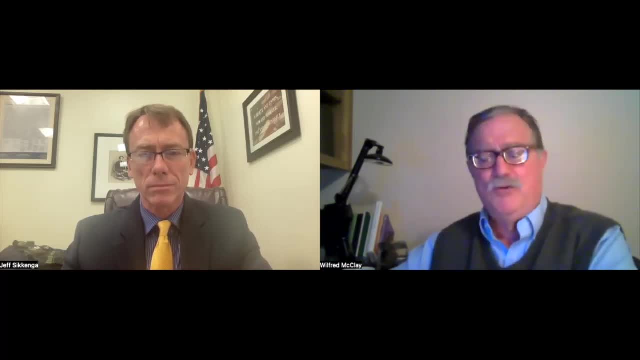 But we do know that he read. Parson Weems' biography of George Washington, which was published in 1799, right after Washington's death- Is often the sort of the platonic ideal in the mind of historians of an unreliable 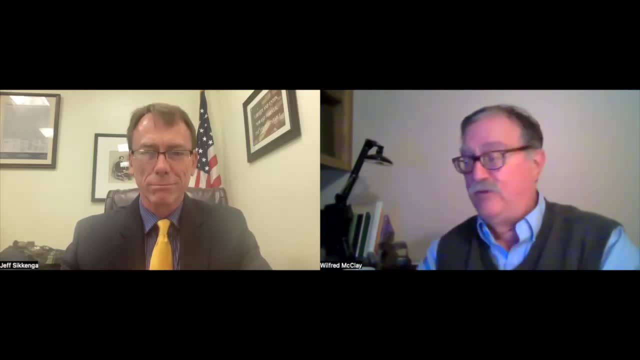 hagiographical work of history. And you know, of course, the famous story about Washington chopping down the cherry tree and admitting to it because he couldn't- he could not lie, and a sign of his, his virtuousness, that he, that he was honest. 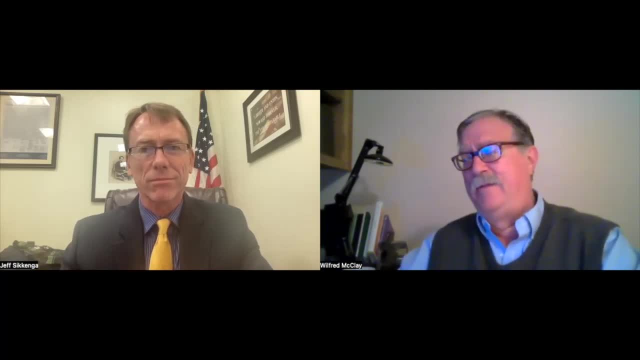 But there's more to the book than that, And Lincoln read it. He remembered it, And 40 years later he's been elected president- Not yet It's been inaugurated. He's traveling across the country to from Springfield to Washington to accept his position. 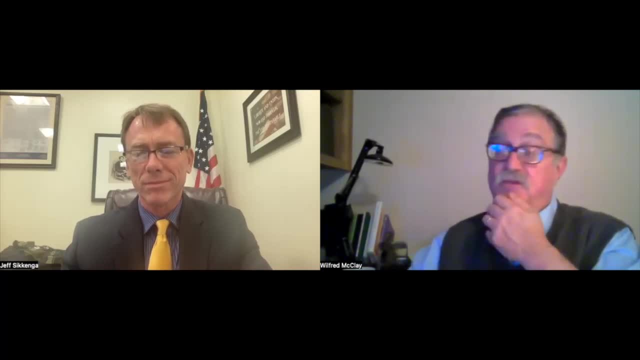 And he stops over in New Jersey, in Trenton, and gives a speech both to the lower and upper houses of Trenton, of the New Jersey legislature, And the one speech to the Senate is the one that that I referenced because he it's very short. 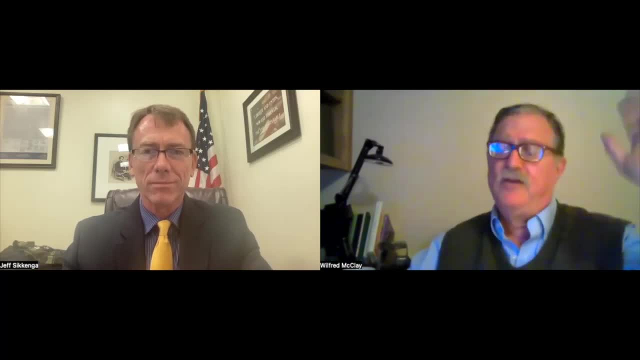 Very short speech But he says, you know, I paraphrase here I don't have Lincoln's gifts of fiction. He says, You know, it's really great to be here Because I remember reading as a young man, as a young boy, about 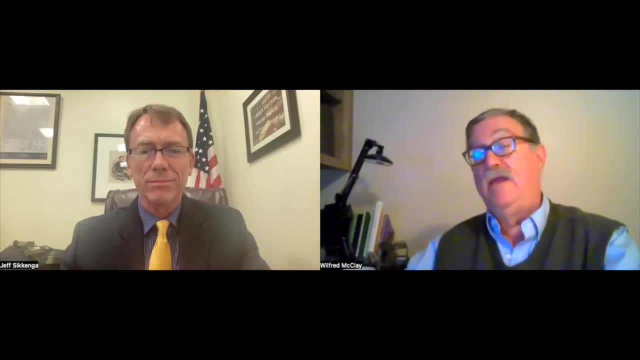 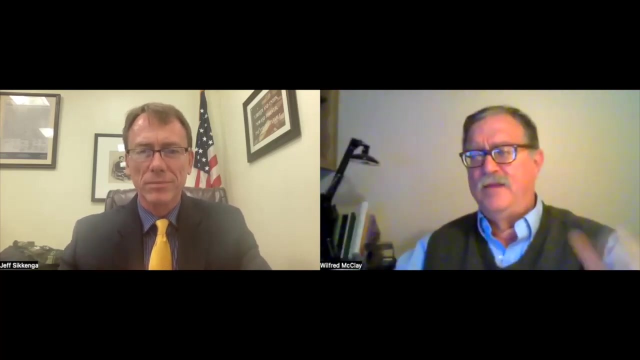 the, the exploits of Americans in the battles, the famous important battles, especially the battle at Trenton, And And all that was entailed, and he goes through a short list of descriptive details about the Hessians and the heated battles and so on. 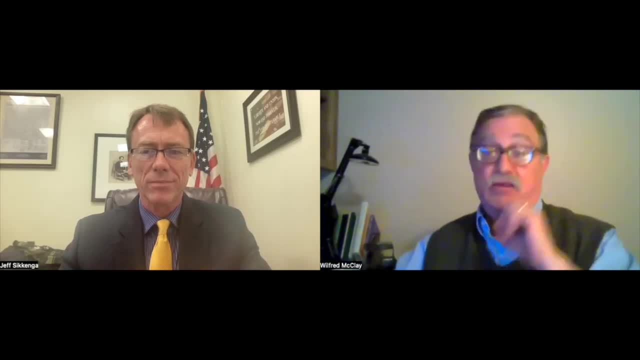 And then he says this: I realized, even as a young boy, that something more was at stake than just winning a battle. Something more was at stake even than the vindication of the revolutionary cause, That it was something that would carry a meaning for all of humanity, for all time. 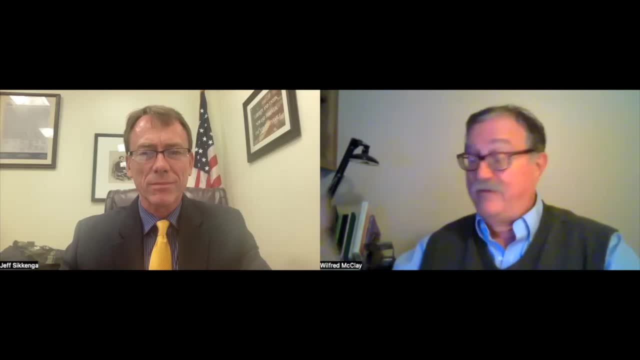 And now you know, you could say, you could be cynical and say as most of my colleagues are, and say, well, sure, he's in New Jersey, He's speaking to the New Jersey legislature, He's going to say that what happened here in Brenton was the most important thing in all of human history. 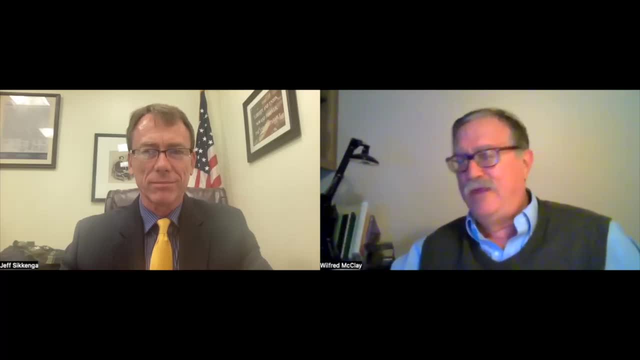 Well, okay, But he didn't say anything at all And what he said was entirely believable. He did remember the book. He did remember the book And my point about that is that this story about the Battle of Trenton, about the heroism of the revolutionary patriots at a time when their back was to the wall, stuck with him and gave him strength, gave him encouragement and courage. 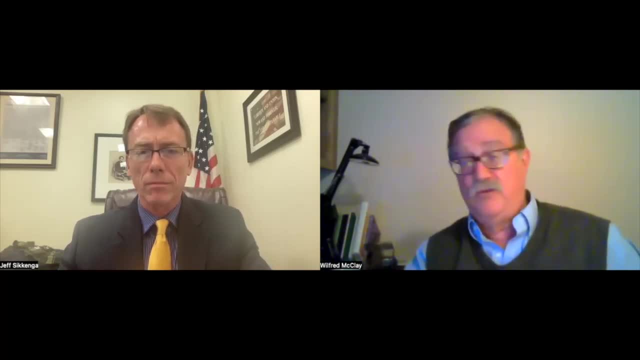 To face the challenge that he was facing, which was much worse in some ways, that, as he was making that trip to Washington, the southern states were seceding left and right. There's reason to wonder whether it would be a country there by the time. you know, March rolled around and he's inaugurating. 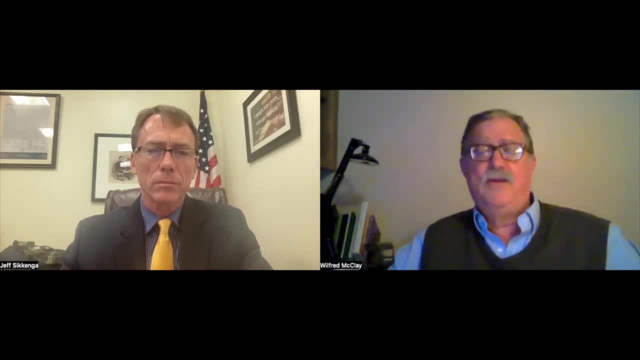 So it's it's. that's a really wonderful example. I'm so glad you brought it up. You have a wonderful example of the way that a knowledge of the past doesn't have to be a dry academic exercise or an exercise in national self-flagellation. 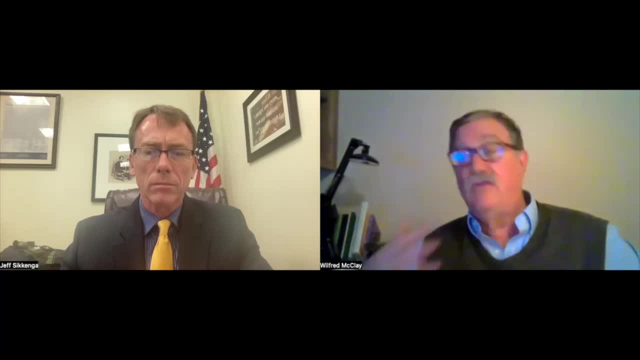 It also can be a source of strength, a source of insight, a source of wisdom, a source of energy and encouragement, helping us to see that the people of the past have faced of our past have faced enormous challenges And yet been able to overcome them. 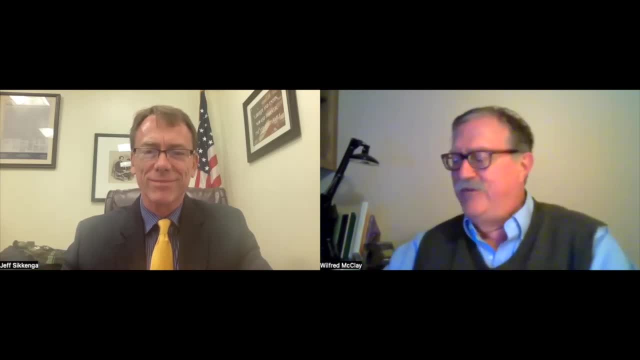 And that's, I think, exactly the kind of thing that young people today need to hear. They need to hear that we've done it before, We've beaten the odds before. They don't need to have a sugar-coated version of the history. 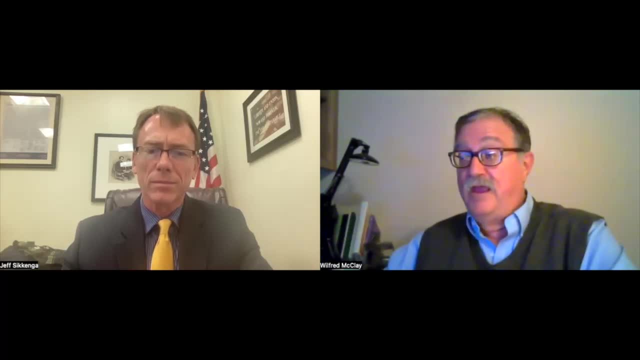 to nevertheless get that point. And we can do it again. We can do it again, We can pull together. Lincoln said- and he wasn't the only one, Lots of people have said this: If America falls, it won't be from an external enemy. 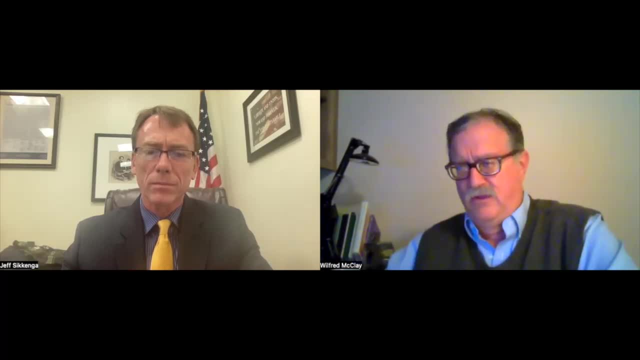 It'll be an internal dissolution, We will lose our own cohesion, We'll lose faith in ourselves, And that, I think, is one of the great challenges of right now. I think that, and I do think maleducation in civics has been a contributing factor. 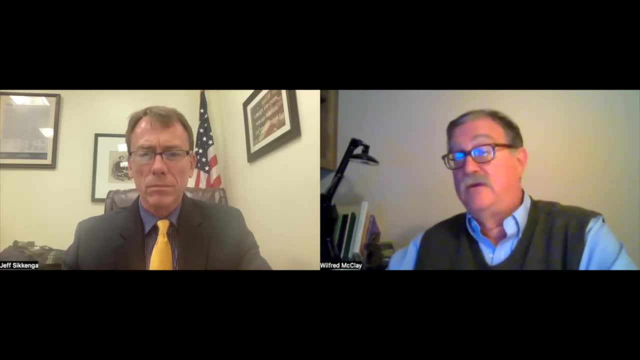 I don't want to attribute too much importance, exaggerate it, but I also don't want to neglect the importance of this. I often think- and here's where I can be accused of exaggerating that, but I'm going to go ahead anyway. 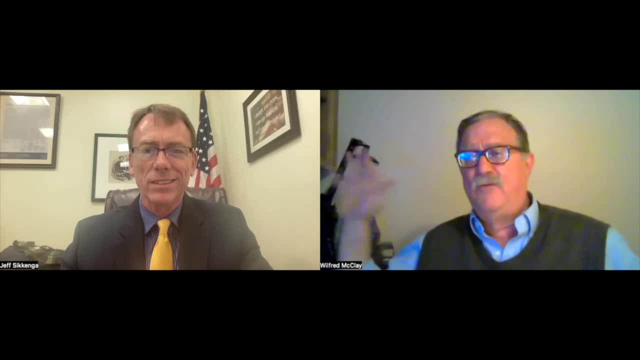 is if you look at the statistics for suicides, for various forms of mental illness, drug abuse, alcohol abuse, opioid deaths, et cetera, that just keep going up and up and up, and particularly for younger people. You look at the sense of discouragement. 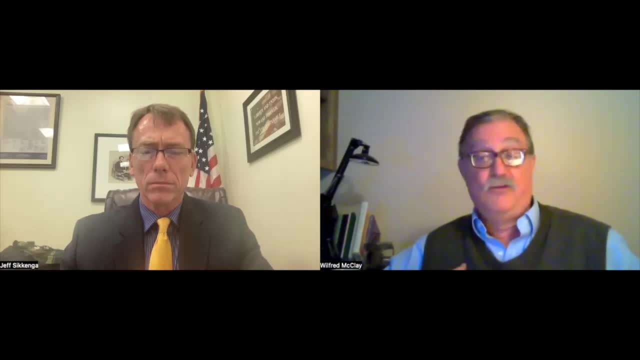 and I teach them and I have to say our students at Hilton College or Joy teach. you don't see a lot of that kind of thing here, but I certainly did. among other places I thought: And that's wrong, That shouldn't be happening. 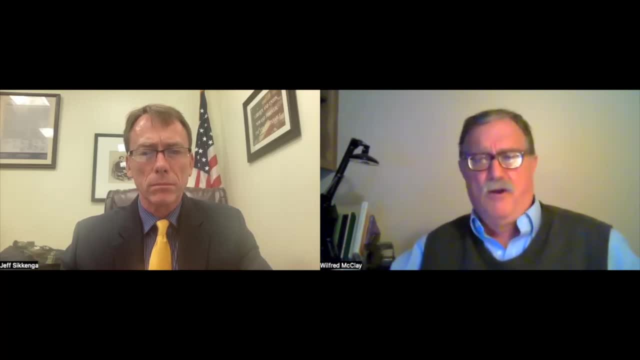 This is still a language. This is still a language. This is still a language of opportunity. This is still a remarkably prosperous country in which there is plenty of room, or plenty of scope, for individual ambition to realize itself. We have a tremendous amount of freedom. which we regularly abuse. Isn't that what freedom's for? to abuse it? But seriously, that it's abused is a sign that we have it, And I think it's frivolous. It's unserious to imagine we'd be better off without it. 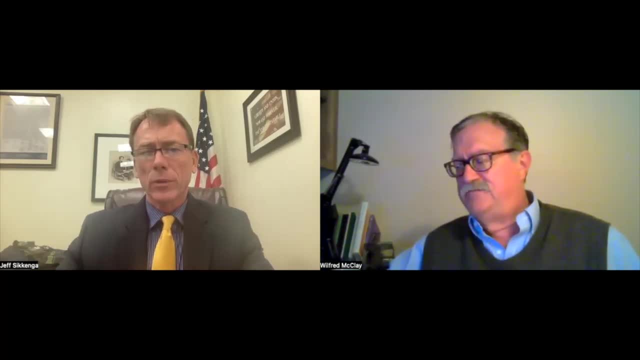 That's really part of the core of what we are. To me it's really interesting, Bill, that you say that, because we run high school programs here at Ashbrook, summer academies where we bring in high school students And one of them we call is telling America's story. 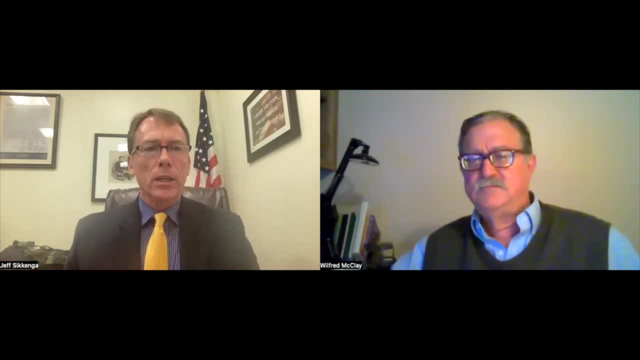 And it strikes me in my experience with those students that when they start to hear the story of America and founding of self-government and a crisis of self-government with people like Abraham Lincoln and then the struggle to sort of fulfill American self-government in the 20th century, they start to see themselves in a way. 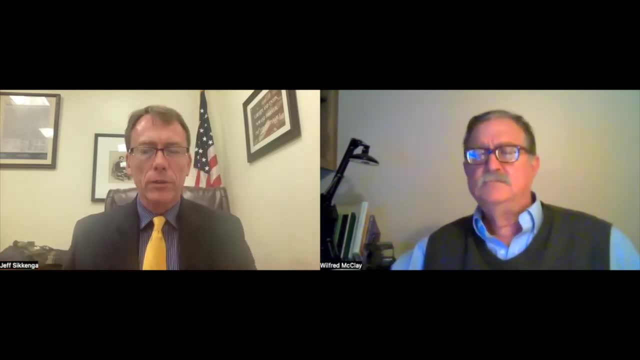 as you said, connected to a larger enterprise. That's a that is not without blemishes but has a kind of it's morally inspiring. It's uplifting to them to hear that story and to know it's not just a bunch of random facts or not just all blemishes. 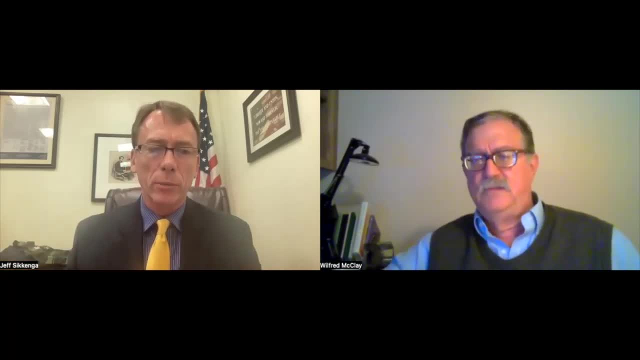 but part of a larger thing That has meaning and makes some sense for them as young people. And I wanted to ask you, because you call your book Land of Hope an invitation to the great American story- Why do you think it's so important to teach civic education? 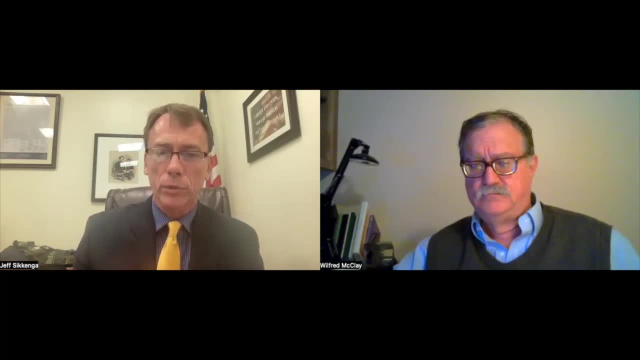 through story, the kind of stories that Lincoln learned when he read Parson Weems. Well, I think that stories and stories are the way we explain the world to ourselves Ultimately. you know it's and the stories are. you know. one of the great things about stories is they can carry. 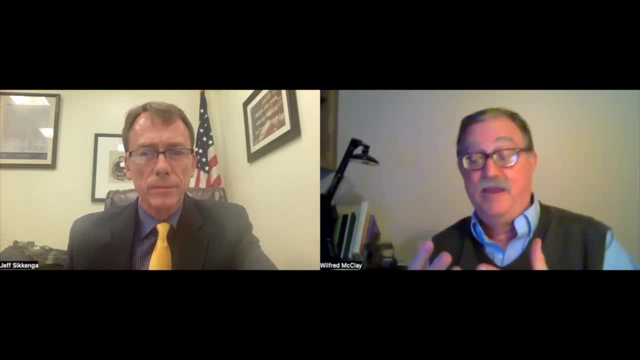 a lot of details and a lot of complexity in them. You can. you can tell a story. that's a complicated story and yet a true story. But think of, for example, just think of- everyday speech. You know, we say, You know, you and I are together and we encounter. 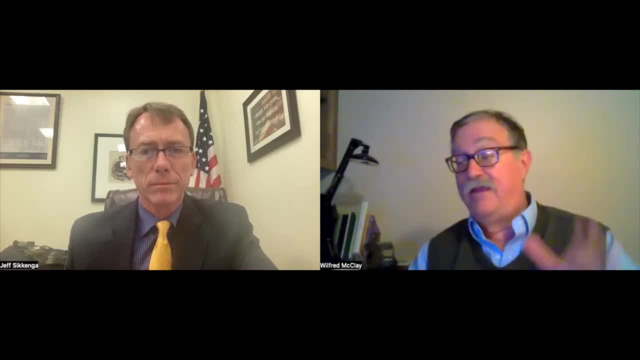 an odd person with odd opinions And he walks away and you look at me and say what's his story? You know- and it really does I- the identity of this man, this peculiar man. there's an implication there that the only way to understand who he is is going to be: 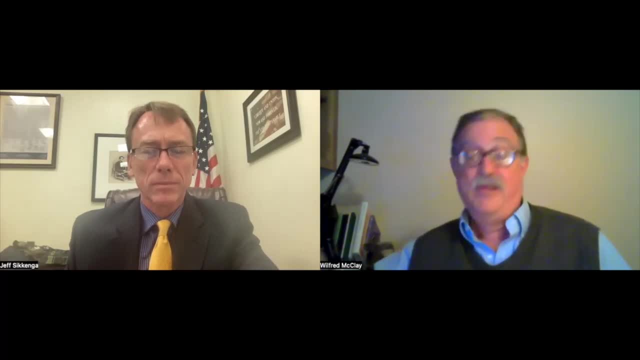 to tell his story and tell a story about him. well, he was, you know, he's brought up this way and he moved from here to there and you know, and it's, uh, you know, fill in the details, but uh, uh, it, it's in some way in which story? and 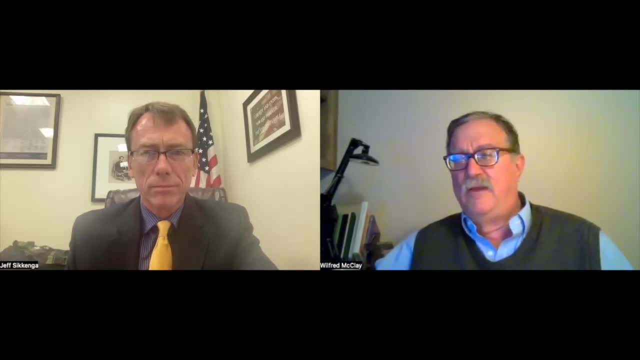 identity are uh are joined, and i think it's important with america, because in america- here's a another analogy i've used uh is that when people have uh- you know, i'm on the semi quintennial commission of the government and it's a very difficult to get any progress because 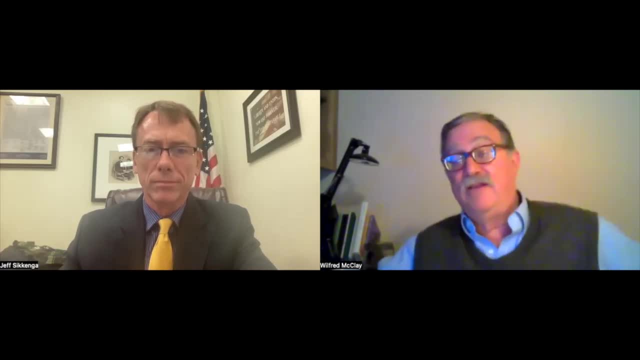 everybody wants to have only their side of things reflected and i have appealed- i don't think with much success- to uh people on the commission saying, look, we should think of the 2050th anniversary of the country as being something like a reunion of one of those huge families. um and um, you know. 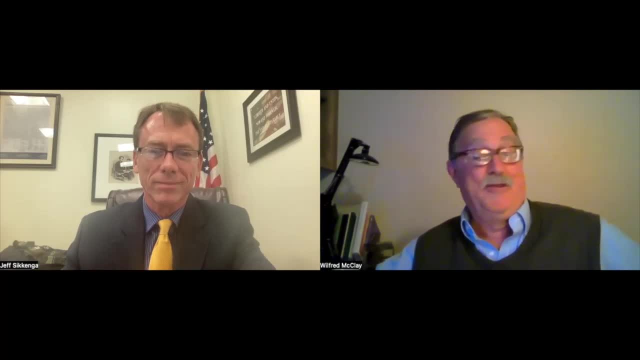 the smiths of, uh, the southeast, uh, united states. they all gather at some place. there's like a thousand of the two thousand. you know it's a huge family. um, most everybody knows, or at least knows of everybody else they sort out. you know, the, the people who are politics are different. 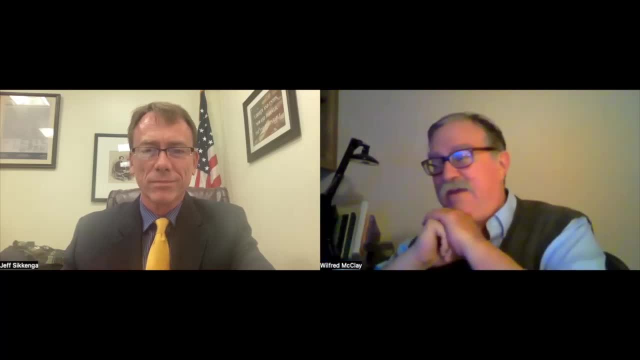 are over here and over here, um, the, the people who, uh, you know, went through the divorce or the separation or the family feud or whatever. um, that's all reflected, but there's a larger umbrella story of being the smith family, that they're all there, even with all their gripes against one another. 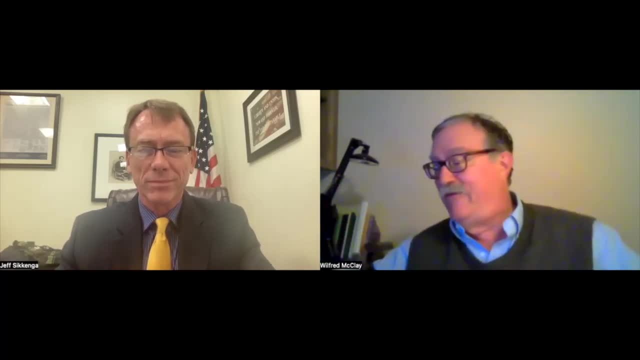 even with all their wounded pride, even with all their sense of uh, of being um, uh, uh, unfairly judged by the others, uh, or in themselves unfairly judging others. even with all that, there's still a story, and i i think that's an interesting way to think about: um, the united. 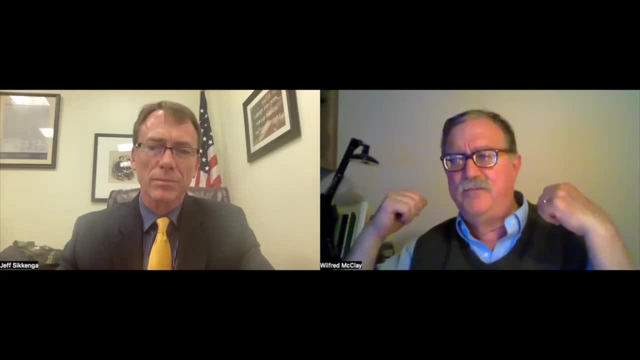 states. we're, we're, we're kind of on a journey together, um, through time. um, we've been through almost a quarter of a millennium- that's a lot of time- um, and with the same constitution most of that time. uh, what, uh, you know what are the commonalities that we have? 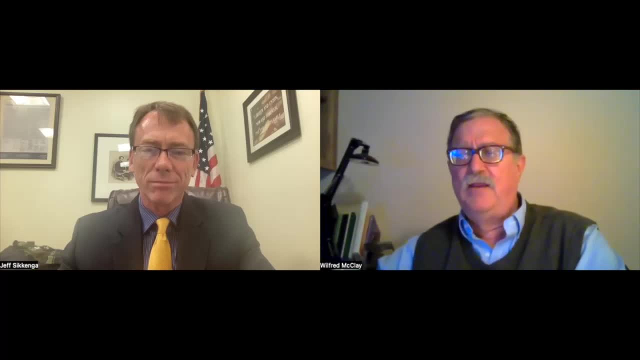 that's um one trend. i may be getting a little off the subject here, but the one trend in civic education has been to emphasize diversity. i've seen this: uh, there's a state i won't name, but i'm evaluating their, their social studies standards, and it's just, there's no indication. 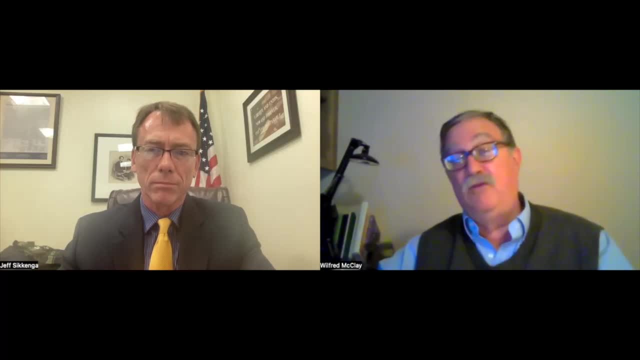 that any. we have anything in common other than this immense amount of diversity, and this is not only debilitating, it's wrong, it's simply wrong. of course, we have much in common. we have this enormous amount in common, and young people shouldn't be taught about diversity without being taught about unity or without being taught about. 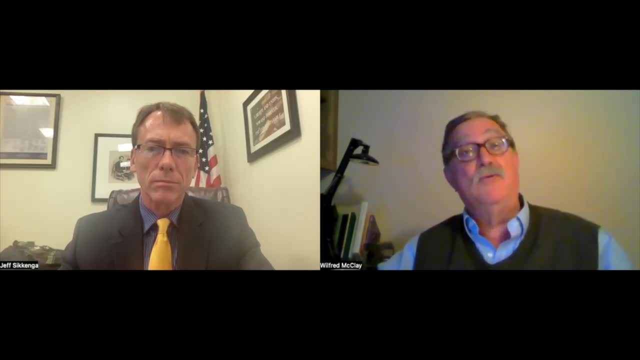 you know commonalities without being taught about membership? that's a word that means a lot to me. is that that sharing membership in the same society? so i, i, um, um, you know that's really. i don't think i need to beat that, but that horse. 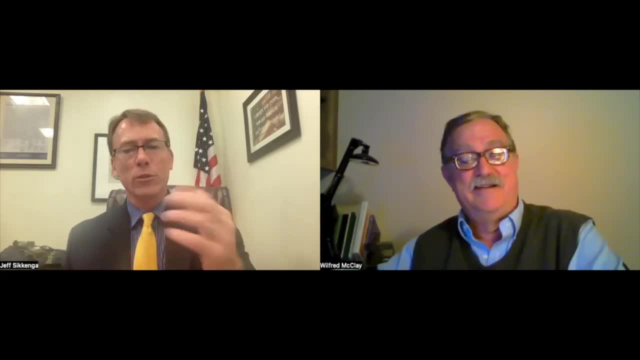 anymore. but you get what i'm saying? sure, absolutely, and that's a fascinating response. and, of course, we have a number of questions from our listeners, but one following up on this. a questioner asks: um, what do you see then as our common bond, if, if it's a story and there's a 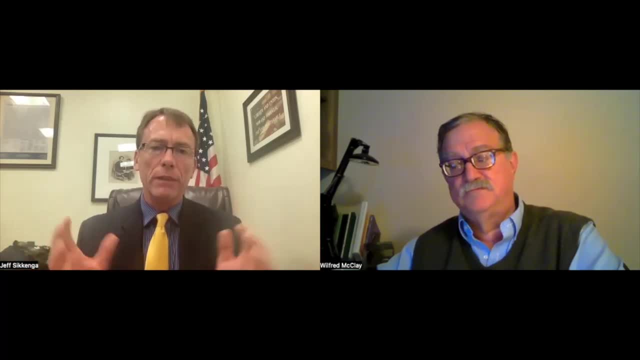 unity, what, what, what are the things that you see in the story that bring americans together as a people? well, uh, and i don't want to be um evasive in answering that question, but but i want to point out that um part of what the question is asking me to do is to extract from the story some propositional 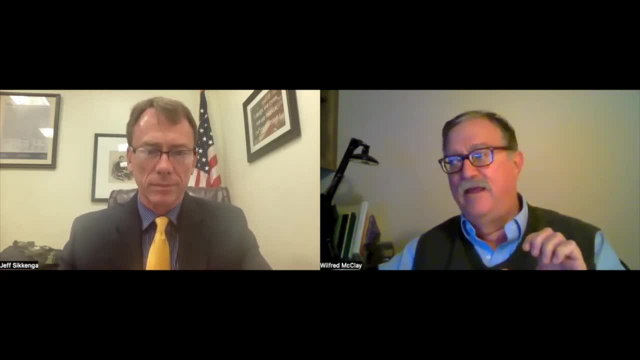 statements about the story and uh, which, in a way, is exactly what the story uh doesn't do. story is not a propositional statement. the story america is about freedom. well, what does that mean, you know? and then we are on a series of propositional statements, um, but okay, having. 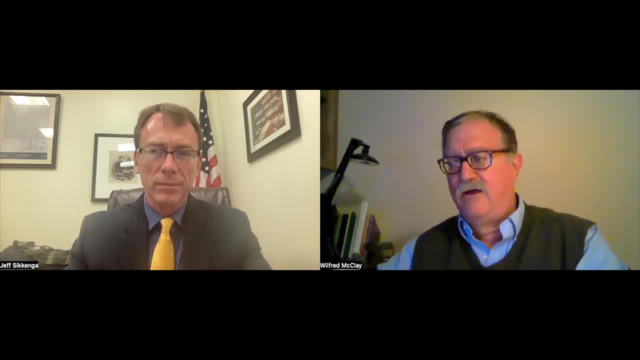 made that minor evasive tactic. i'll. i'll say that, uh, i think there are there's. there are certain values that we share in common, and, of course, one of them is our sense of the value of freedom. one of them is a a uh, an estimate, high estimation of equality, um uh, the, a preference for the ideal of self-government. 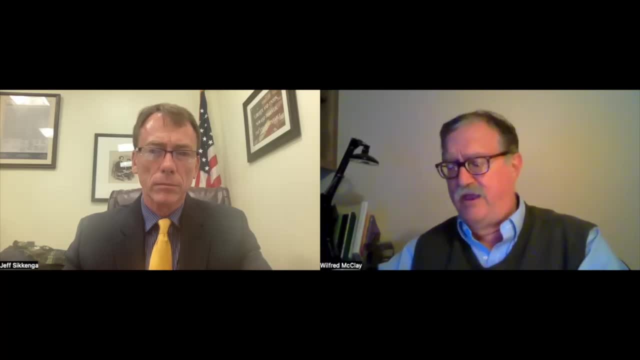 people get to govern themselves, to choose for themselves however they would like to live, um, uh, and respect all the sort of first amendment, um, restrictions on, uh, what, what government can do with regard to speech, with regard to press, with the right assembly? those, those things all i think. 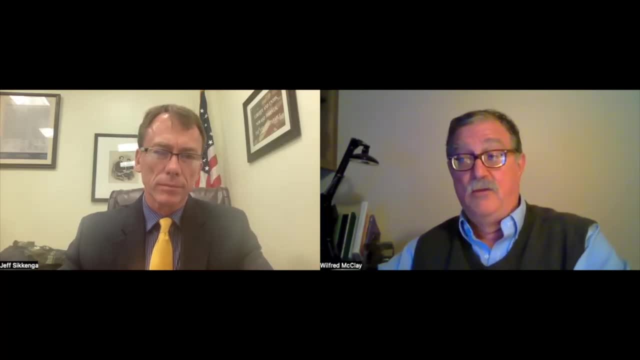 matter enormously to us and to to everybody. um, i, you know, i mean, yes, you could find people who are opposed to freedom of speech, but, um, it's not a, it's not really a serious issue, but it's not a just widespread position. i mean it's not a position widespread as in its serious time. um, 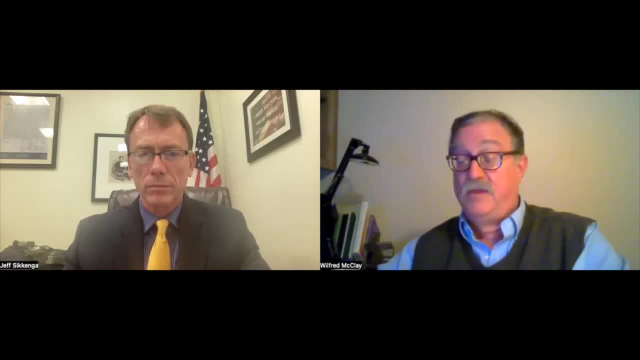 in the press and and so on. freedom of religion, um, now there are people who would like freedom from religion, um, and that's, that's a legitimate point of view, uh, but it's not incompatible with the first amendment, the language first amendment, as it's drafted. so i i think after a lot of the commonalities, 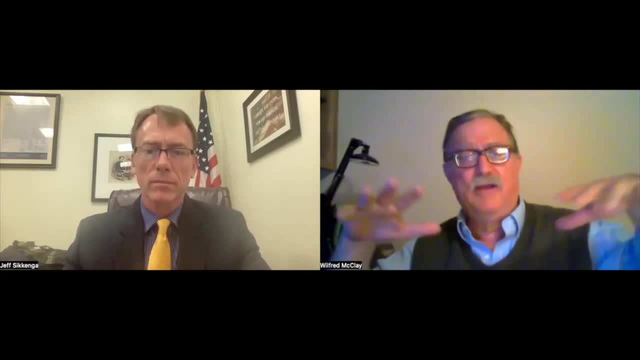 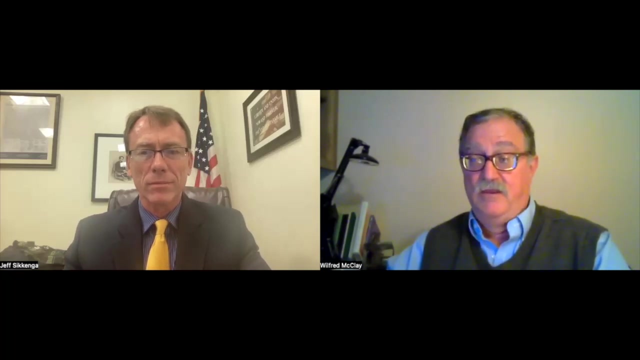 you notice in my answer. i mean a lot of the commonalities drift back towards this constitution and i think one of the reasons i'm so hot to keep the constitution- independentism. i think it's precisely because of our diversity in other ways that we need some rock solid solidities. 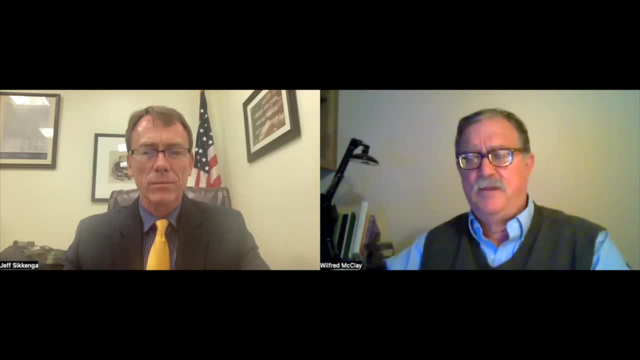 to recur to um, if we're going to have such a remarkably diverse culture, which, you know, there's the diversity of um, all kinds of very fundamental things having to do with lifestyles and um, uh, you know the general philosophical outlook. i still think that the language of the declaration, the, the uh, the opening paragraphs of the declaration. 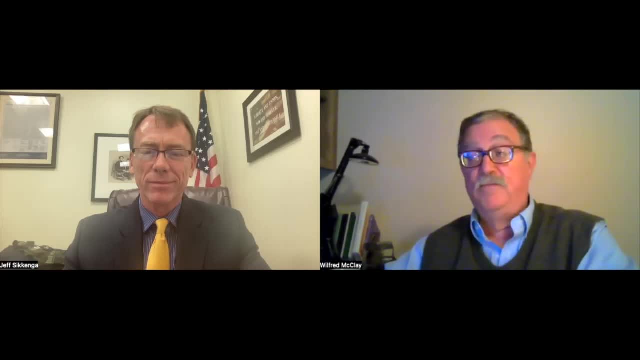 is very surfaceable, where, uh, i don't see anything in there that is likely to be particularly objectionable to to a lot of americans- um, maybe some, because there's always somebody who can object to anything- but but not a widespread objection, i think. uh, i don't think. 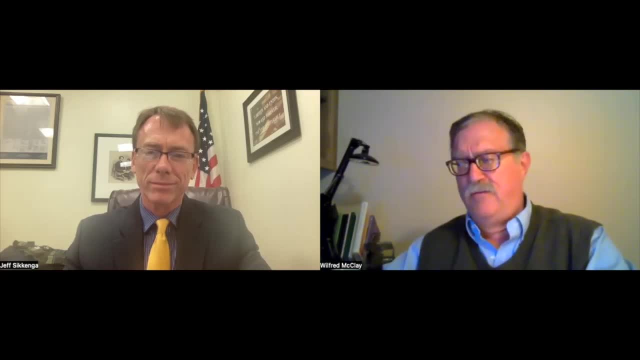 this is as hard, as difficult as we sometimes make it um. one of the best experiences i've ever had was i was a fulbright professor in italy for a year and uh um, and i remember having discussions with my students. i taught graduate students only, and they were um italians. 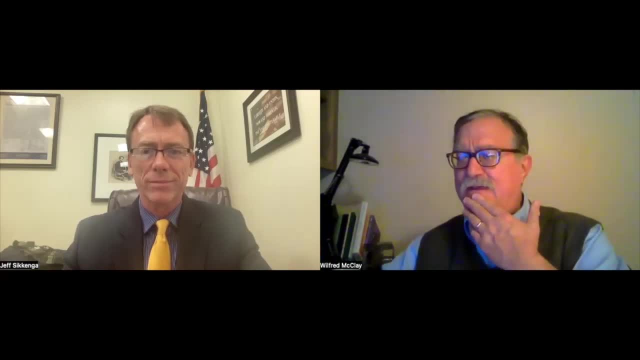 as you may know, are very, still very regional in their mentality. people think of themselves, as you know, being from genoa or tuscany or or whatever, and and um uh, and in fact one class i was talking about. don't you think there's such a thing as italian national character? and one of my 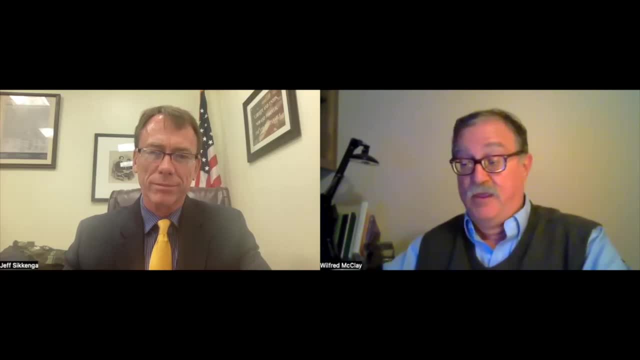 students. a very beloved student i'm still in touch with said: uh, professor mcclay, when i we hear people talk about italia, we assume he's a fascist. so so, italians, the idea of national character is something they're very averse to. but i said: well, would you say the same thing about americans? oh no, 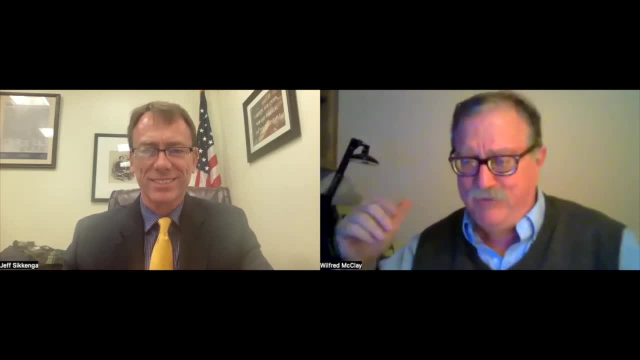 americans. my god, if there's any people on earth that have a national character, you can identify it's americans. i can tell an american walking down the street- uh, yeah, i can tell an american walking down the street- uh, yeah, i can tell an american walking down the street- uh, yeah, i can tell an. 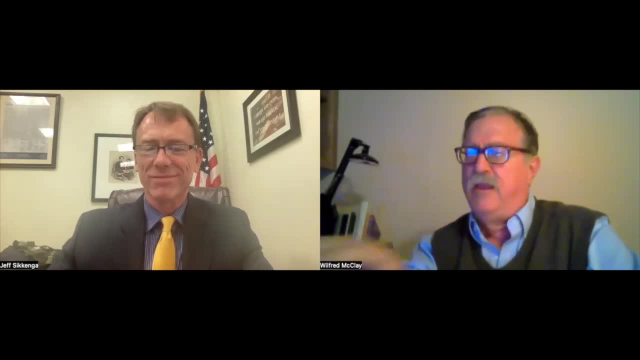 african-american and a nigerian or whatever, just to look at it, just to look at the way he walks, and they insist on this, and i mean anybody who's traveled- i, you, you, in europe, elsewhere you run the same thing. there's something there is an american that there is an americanness about. 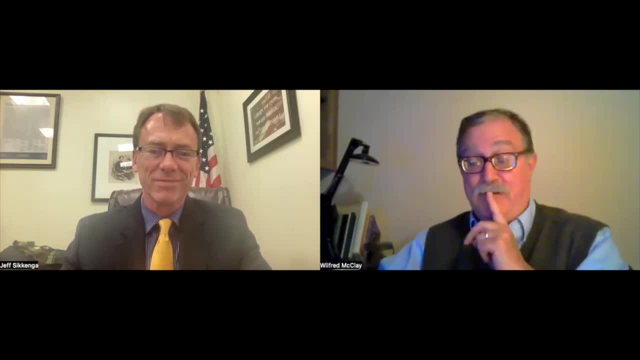 about americans that other people notice. um, it's not easily defined, but, um, it's there and it does seem to me that, um, uh, it would be good for us to understand better. yeah, that's a, that's a worthy admonition, a fascinating story of america, insightful. 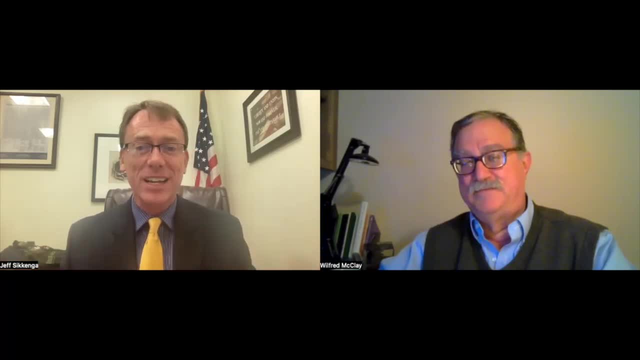 interesting, inspiring, perplexing even sometimes. yeah, absolutely so interesting. that's why i love the title of your book: land of hope. uh, that's a great title. um, bill mcclay, thank you so much for i'm to join you, us for the conversation. uh, really deeply, and let me just say i, i'm a great admirer. i mean, i, i'm 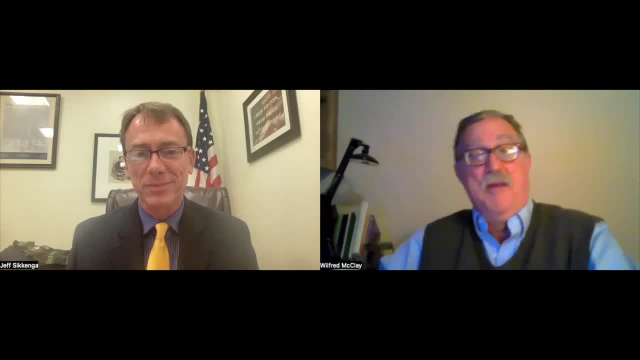 kind of have a conflict of interest here, since i do serve on the board, but i think that for year in and year out, through a succession of leaders, uh ashbrook has been a very important force in, uh in in in dealing with these, these very issues that the need to have a conscious 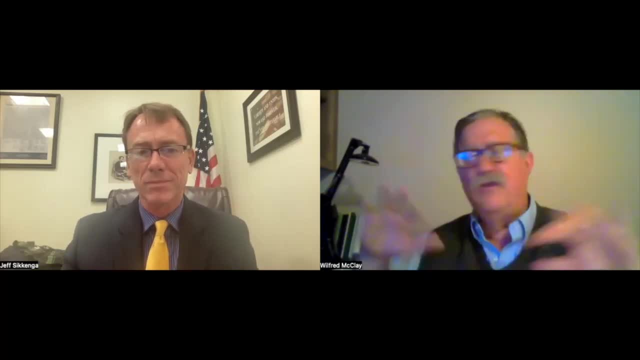 appropriation of the world and the need to have a conscious appropriation of the world, of our heritage, that we can't just waltz into it mindlessly, um, uh, by watching, you know, music videos and playing video games, whatever tick tock, we can't just waltz into a knowledge. 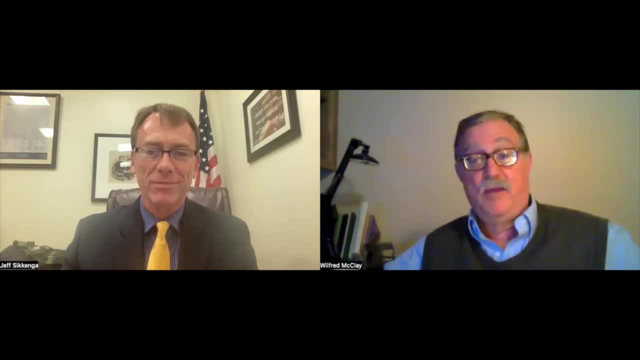 of who and what we are, we have to know, we have to know about the past. there's no such. that is truly what we believe, we, that we need to understand our history and our principles. so, bill, thank you again for taking the time to join us this evening, for our listeners. 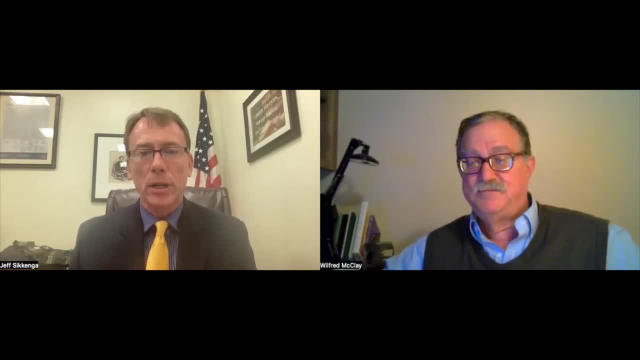 appreciate. if you want to know more about ashbrook, you can look us up online, of course, at ashbrookorg for teachers who may be joining us. you can look at us up us up at teachingamericanhistoryorg or tahorg. uh. those of you who are with us will be sent a link to a recording of this uh conversation. 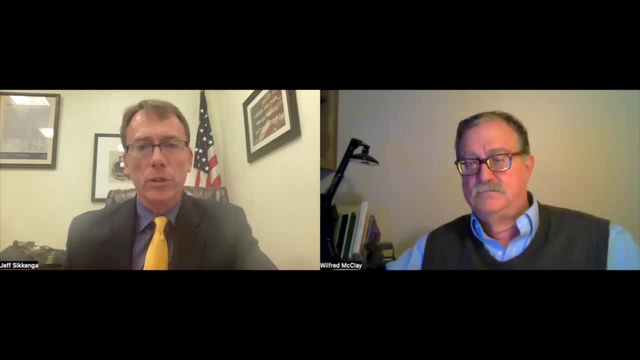 please free to share with your friends, your family, your colleagues. we'd love to get the word out far and wide: the young people in your wife life, your children, your grandchildren, who need to hear this kind of conversation and know the kind of education about america that they should be getting, the kind. 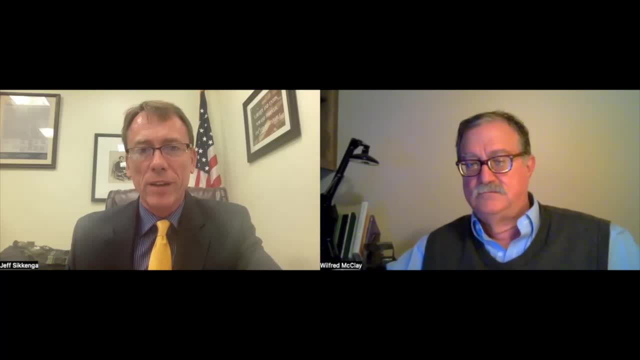 of professor mcclay talked about tonight. we really believe that you have these kind of conversations. they do renew your hope in america. they do renew your hope and the possibility of that kind of education of the heart and mind that professor mcclay was talking about. so again, i want to thank. 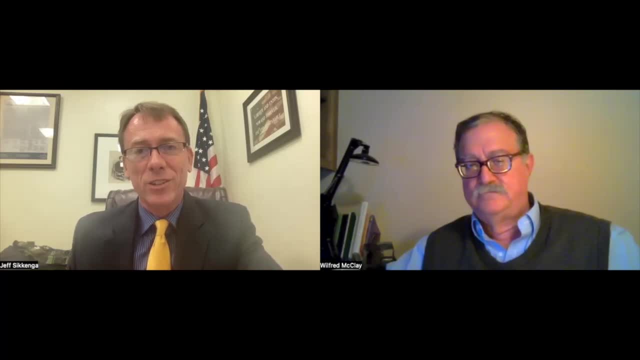 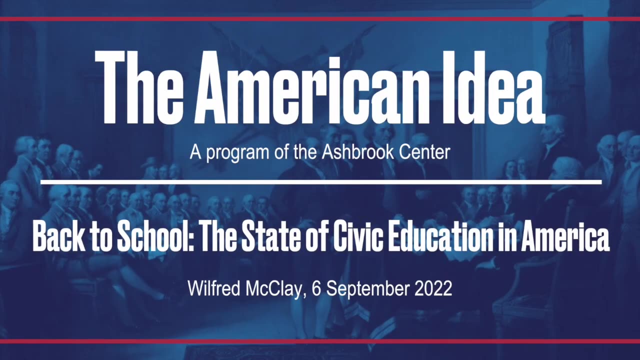 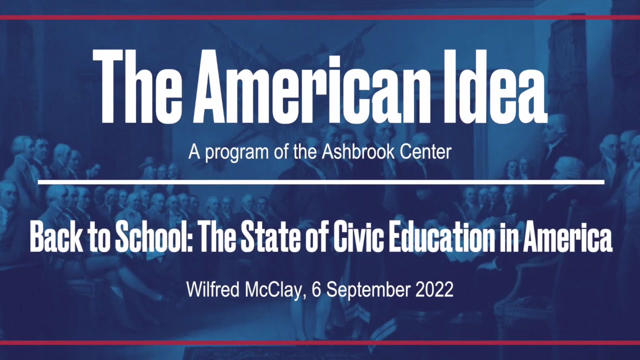 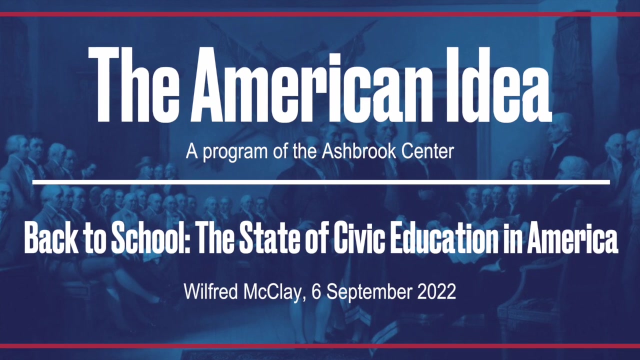 you all for joining us and, as always, we end by saying: stay healthy, stay hopeful and stay connected with ashbrook, thank you. thanks for joining us for this episode of the american idea, a production of the ashbrook center. we're here to explore america's history and principles and what they mean for today. what